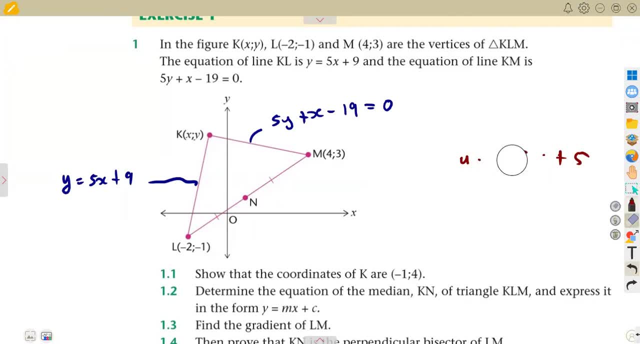 So do not be scared about that equation, the format that you have, where this part we can even make Y the subject. Let us do, you can write the way that you want. 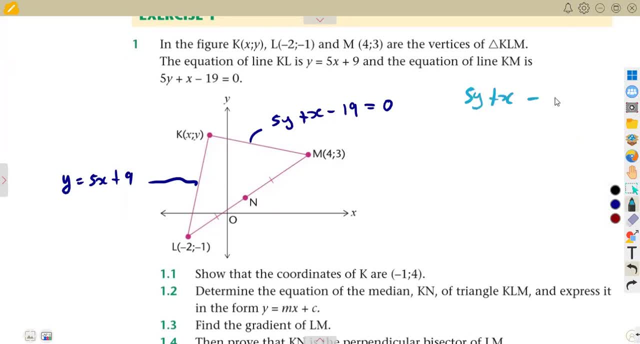 All right, let us see this 5Y plus X minus 19 is equal to 0. We can even transpose those numbers back to where they were before. To the right-hand side, this will be a negative. To the right-hand 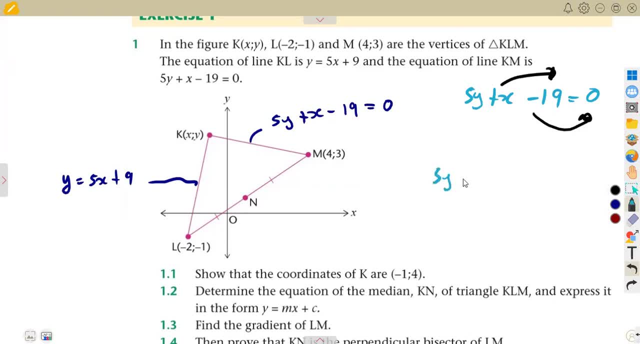 side, this will be a positive. So meaning to say 5Y is equal to minus X plus 19. Remember, 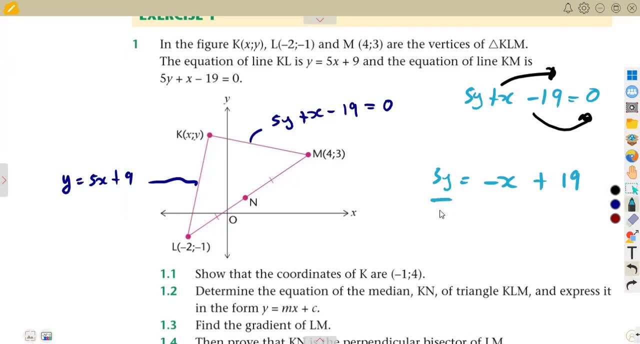 say this is going to be a positive. So if I am to divide by 5, by 5, by 5, each and every term Y is going to be, this is minus X over 5. There is a minus 1 there. 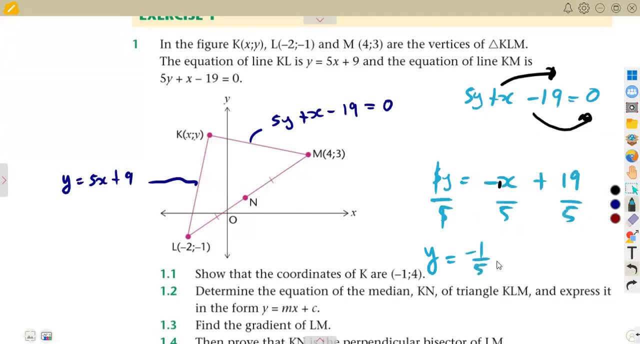 So it is the same as minus 1 over 5X plus 19 over 5. Guys, it is up to you, the way that you solve 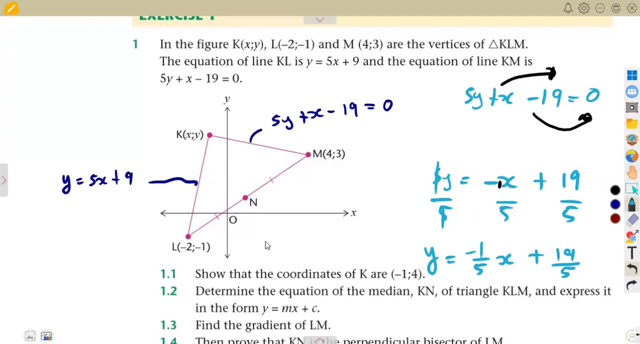 an equation. I mean, the way that you want your equation to be written is, it is up to you. It is up to you. 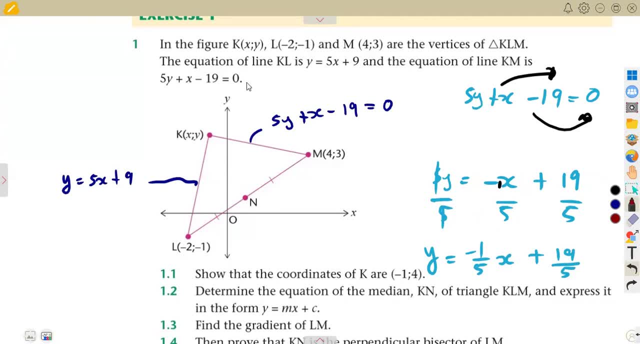 The way that you want this to be written as. All right. So this is not part of our question. 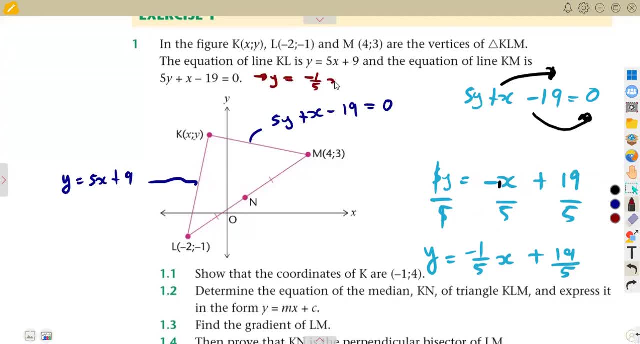 I'm just saying. So it can be written as Y is equal to minus of X plus 19 over 5. So I'm not saying you're supposed to, whenever you see this, you write this. No, no, no, no. I'm saying it is the same thing. Don't be afraid. When you see this format, it's still one of the same format as you 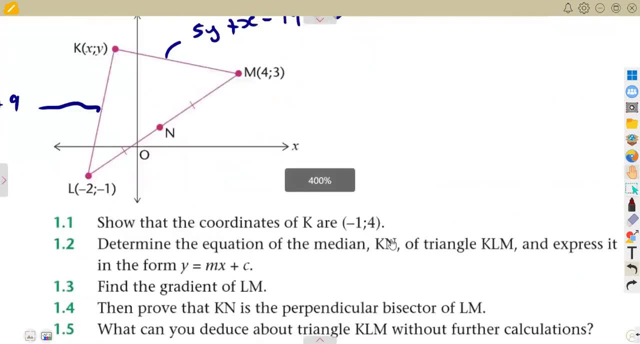 are used to before. All right. So let us answer the first question. Show that the coordinates K is given as minus 1, 4. 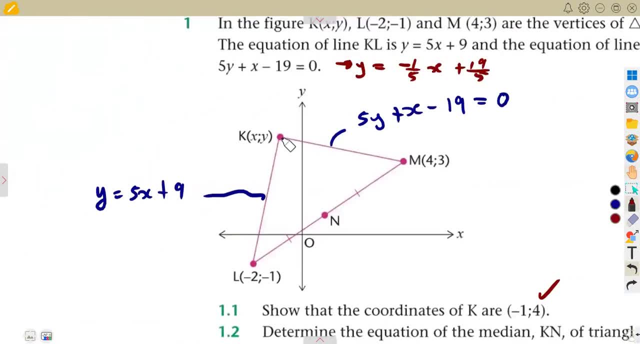 K is this point. And K is the point of intersection of the two lines. So it follows that we never talked about this in our previous class, but let us refer to this. It follows that whenever you refer to the point of intersection. The point of intersection. The point of intersection is the one that you have when two lines intersect, when two lines meet. If you're given two lines, they do meet at a time. So the point of intersection is the point of intersection. 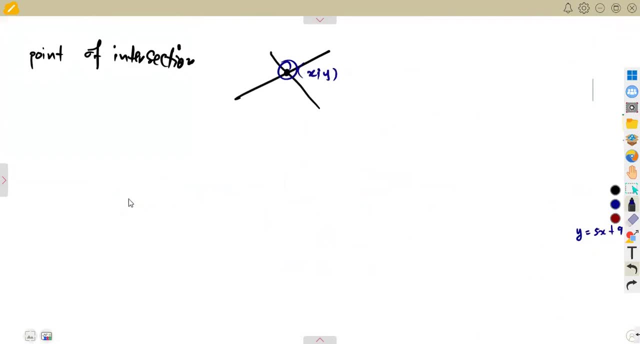 certain point which is referred to as x y remember a point is always x y so to have that point of intersection you simply have to solve the given equation simultaneously give solve all right so 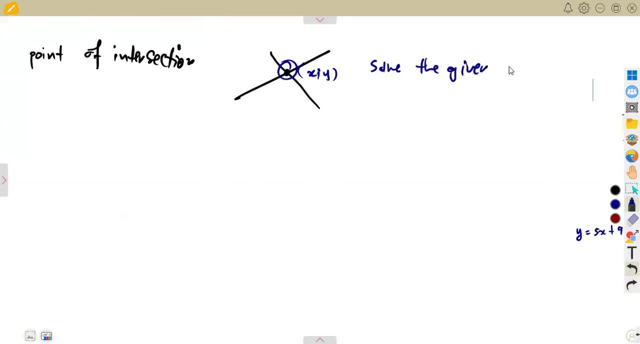 just solve uh the given equations the given equations simultaneously meaning to say we are back to our simultaneous equations remember in simultaneous equations you'll be given two equations then you're asked to solve simultaneously the same way that you're solving those simultaneous equation you're determining x and y at the same time that is 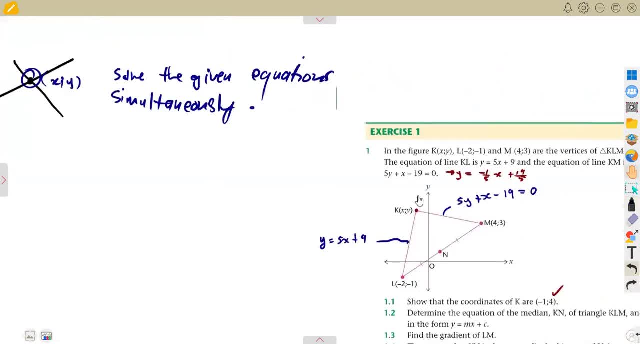 the same way that you're going to have so in this question that you are given on number one we are asked to show that k is minus one four so this is 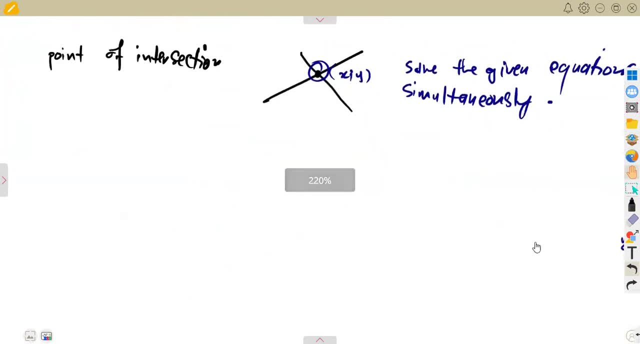 what you're given on question number one we need to show that k is um minus one four so this is our point k that we need we need we need to show this so how can we show this 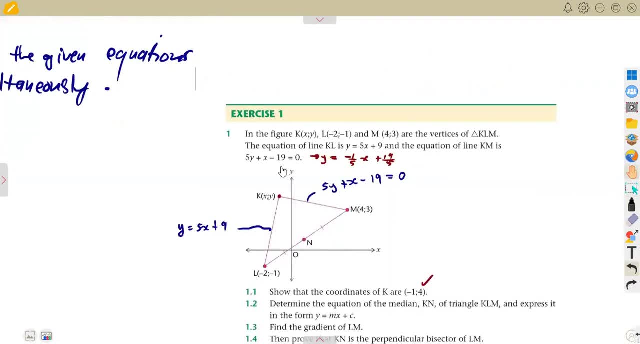 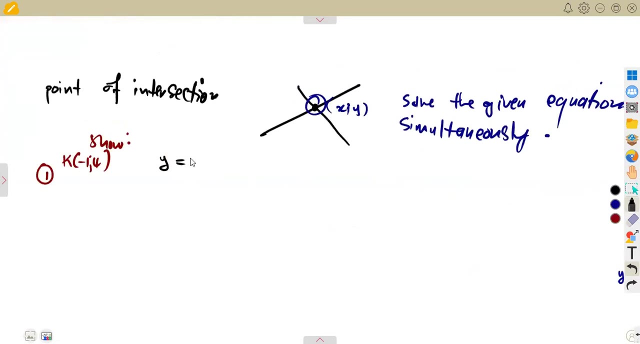 remember we are given the two equations there the equation of this line and also the other line km so we can solve these simultaneously we have the equations of the given lines so like i said you can solve them simultaneously the first line is given as y is equal to 5x plus 9 remember from 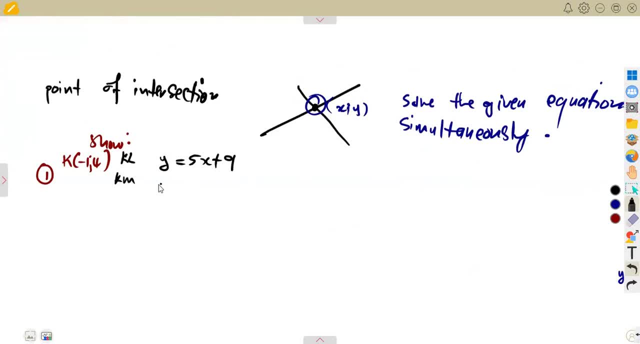 our line kl then also the line km we are given this as 5y plus x minus 19 which is equal to 0 so we are going to solve these two equations simultaneously i've got the first equation 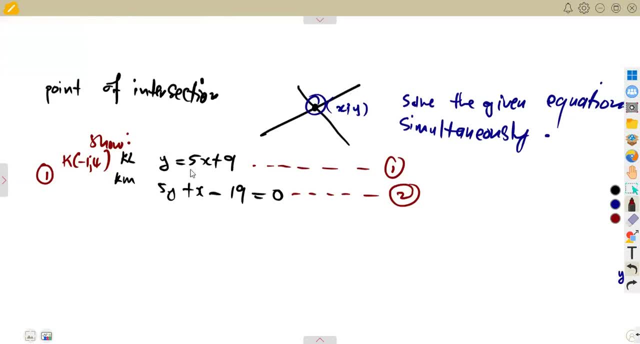 and i also have the second equation so taking advantage of the first equation that y is already the subject of the formula 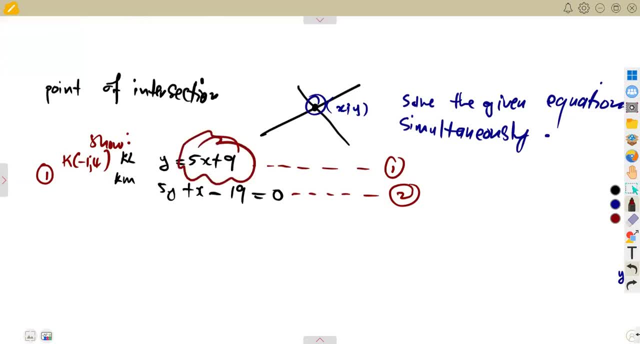 y is written in terms of x so what i can just do is to substitute equation one into two all right 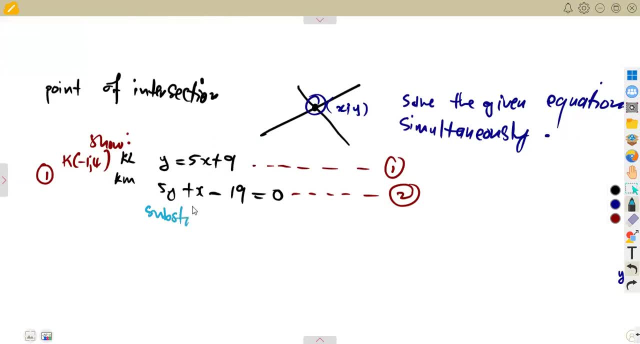 by using substitution method i'm going to substitute all right equation one into two 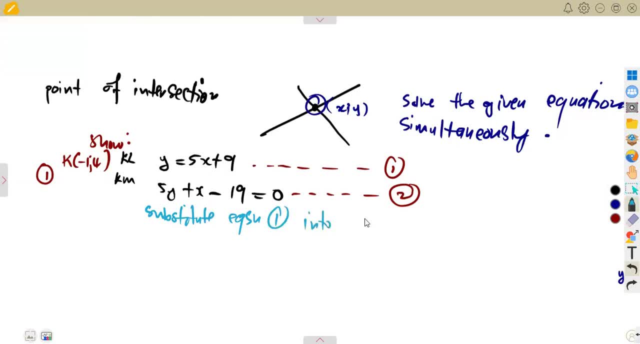 so in short that's equation one into equation two so that is y in place of what uh where there's a y 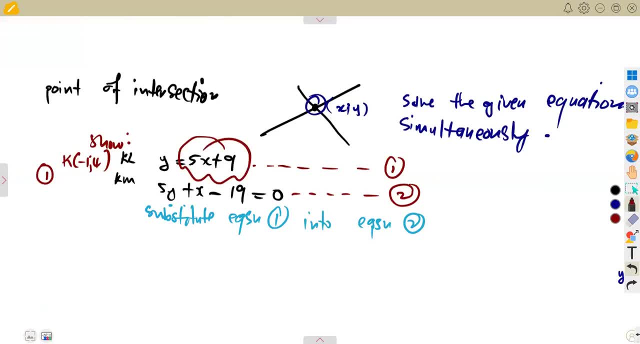 they're going to substitute what is represented there in terms of what in terms of x remember 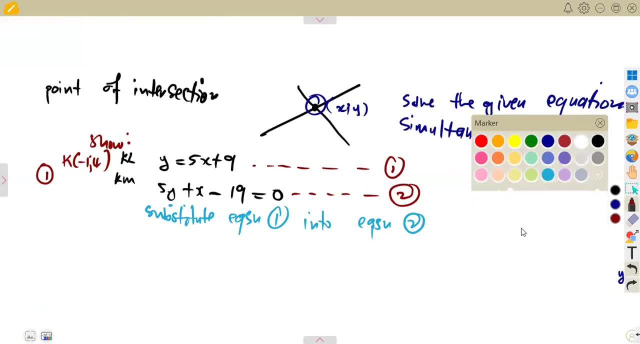 that we are given that y is equal to 5x uh plus 9. this part here is the one that you need to substitute where there 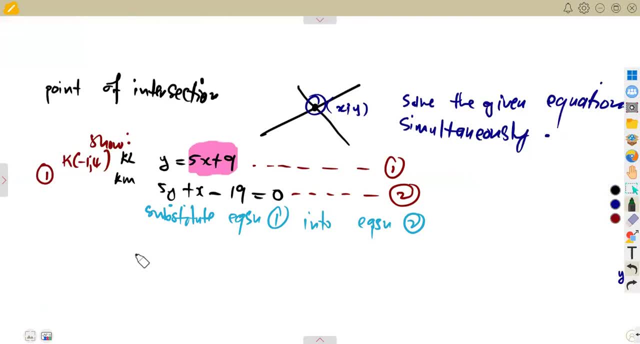 is a y in the second equation all right so let us consider this that is going to be five times 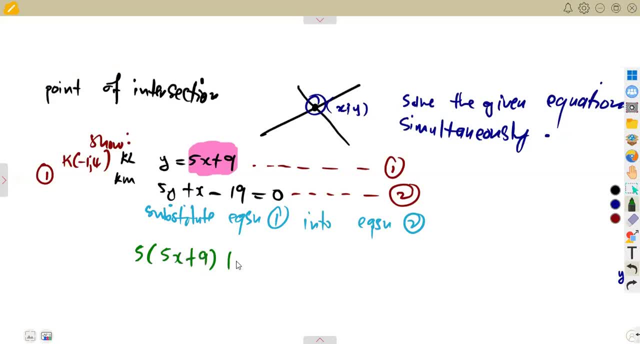 in place of y you're going to substitute 5x plus 9 plus x x is there's nothing to be substituted for x 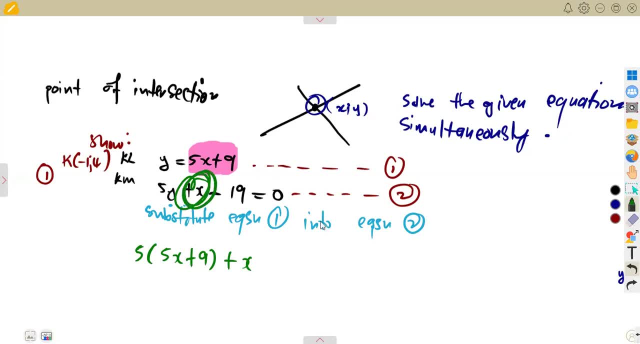 it is the part of y that is affected x remains as it is it is not affected all right 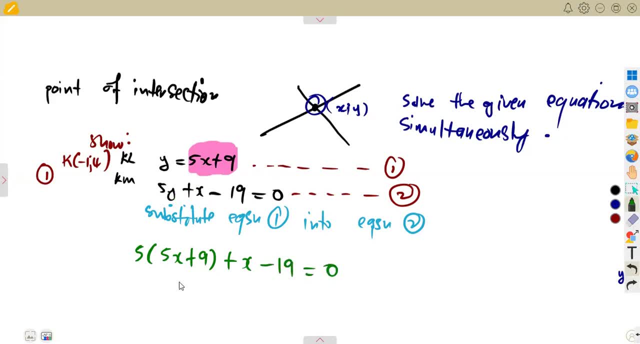 so that is minus 19 is equal to 0. so expand by 5 what are we going to have that is uh 25x plus 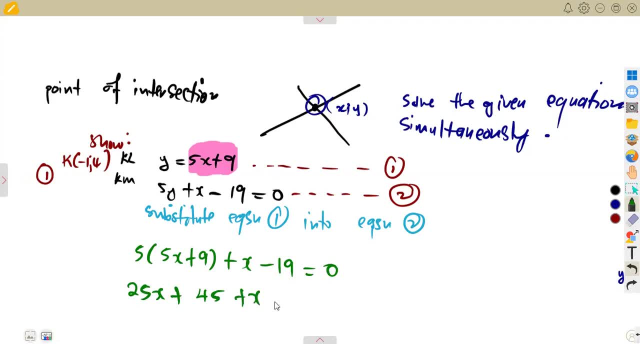 5 times 9 which is 45 uh plus x minus 19 is equal to a 0. so solving this equation we can see that 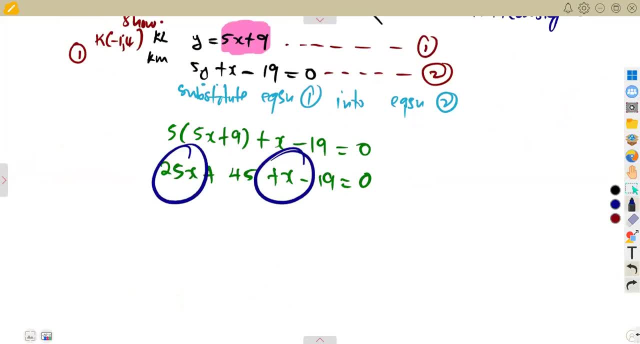 we've got like terms the part of x the part of x so we are going to collect uh the like terms in 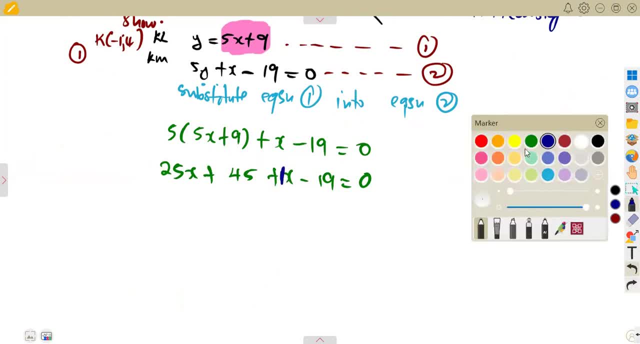 this case this is the same as there is a one x so let us add 25 plus one that is 26 x okay 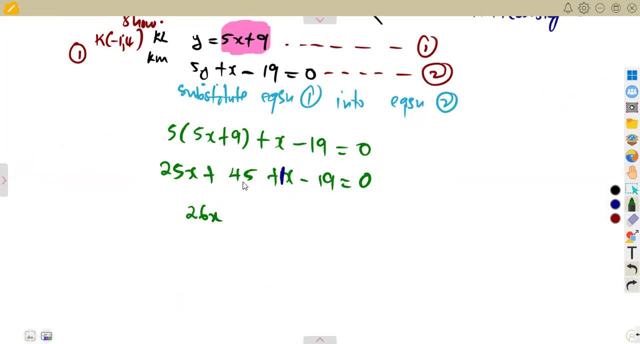 the part also of these numbers you can subtract uh 45 minus 19 uh that is going to be a positive 26 and this is um that is equal to 0 so transposing a negative i mean the positive 26 is going to be 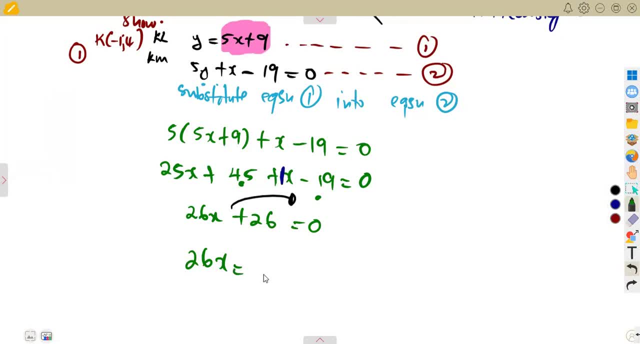 a negative 26 on the right hand side so this will be negative 26 so let's divide guys by 26 let's see what are we going to have at the end our x value will be a negative one uh so that 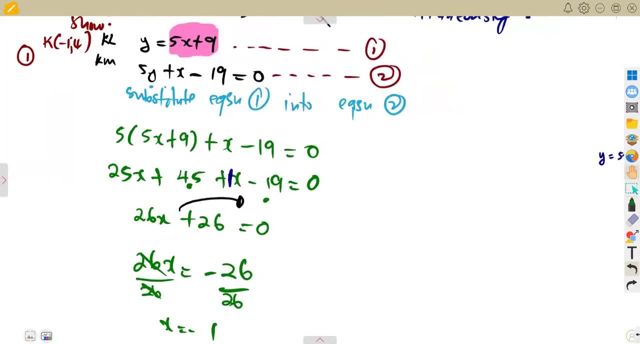 means we can determine the y value by substituting in any of these two equations in any of these three but i can take also advantage of the first equation because already y is the subject y is equal to 5x plus 9 so you can simply substitute the x value and determine uh the y value so that is 5 times x remember our x is negative 1 plus 9 so that is going to give us a positive 4 at the end minus 5 plus 9 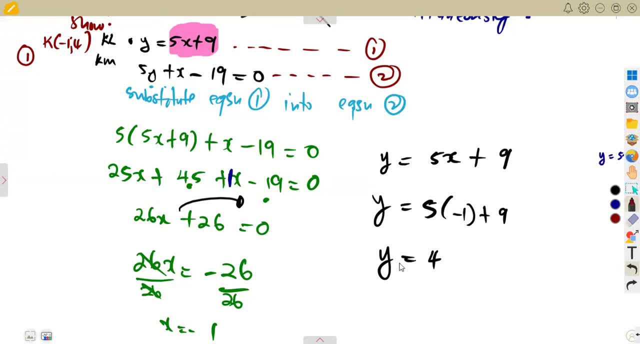 that is a positive form so as you can see that's exactly the k that we wanted in this case minus 1 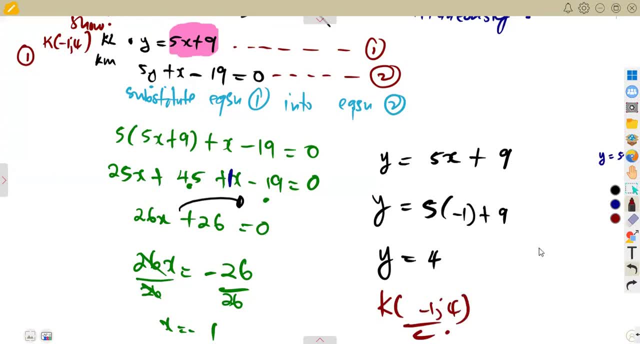 4 the x value to the y value so this is what you're being asked to show so that is exactly what we obtained there so be careful so this one is fine so meaning to say our k here is minus 1 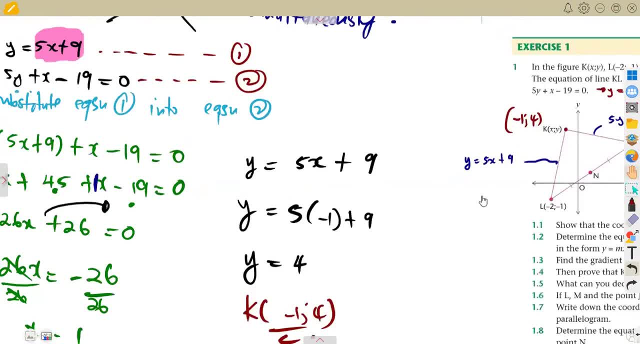 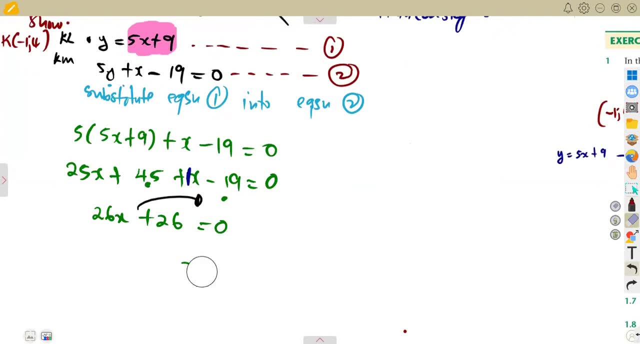 4 that is what we have at point k all right so uh just for the sake of uh having our persons next to the diagram let us just remove this i just hope we are clear on this one uh so let us revise as much questions as we can uh meds is not that difficult uh if you are someone 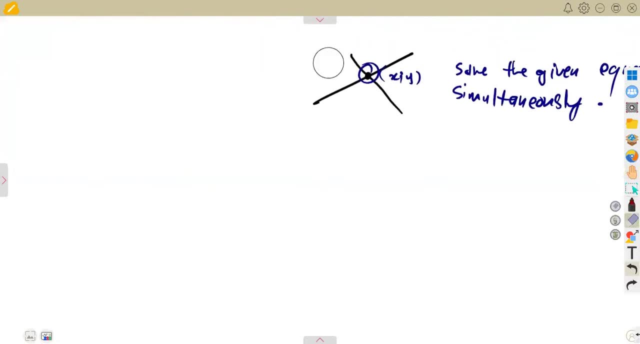 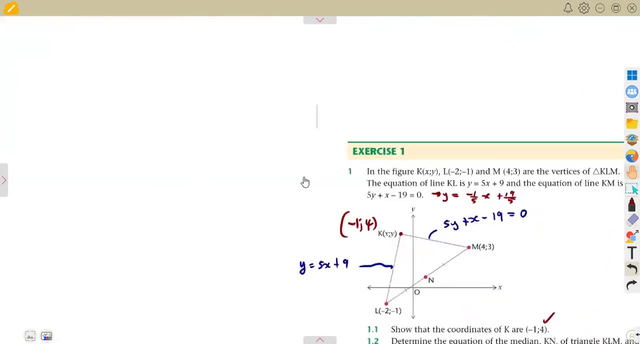 who is working this on a daily basis and also doing question papers after each and every introduction you do revisions on question papers you see that meds is not that difficult 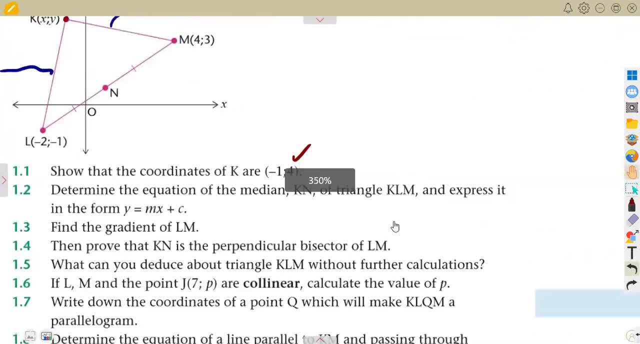 uh it is just a repetition uh it is just a follow-up it is just something that is just like a pattern it's just like art you see so the more you revise 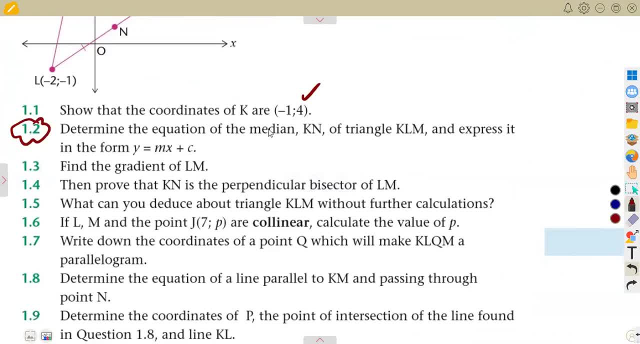 the more it becomes part of you that's it determine the equation of the median k n 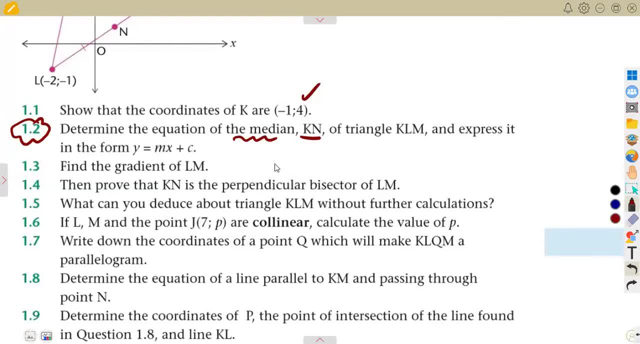 what is a median that is the question of triangle k l m express it in this form which is the format of y is equal to m x plus c we talked about this which is the gradient intercept form we need the equation of the median of the gradient intercept form we need the equation of the median of the 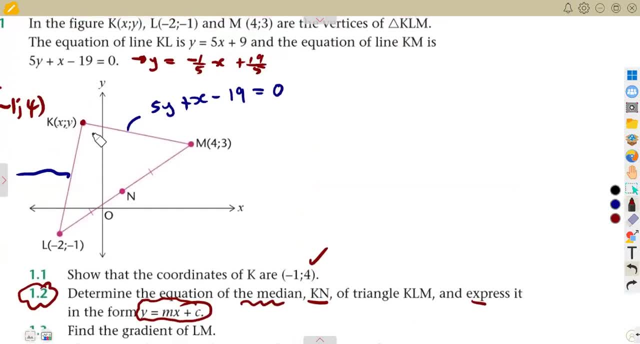 gradient uh k n this is k to n this one k to n the equation of this line so what is happening is that n there is the midpoint for this to be a median line a line 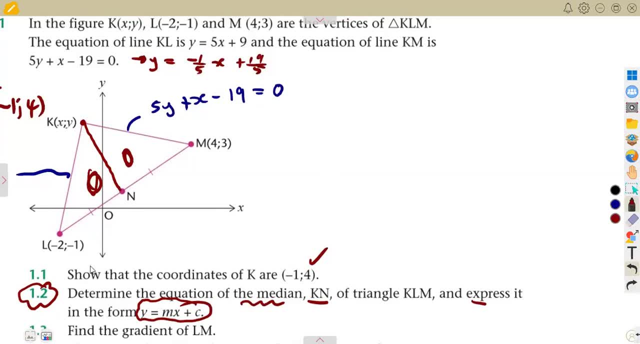 which divides this triangle into two equal paths it means that this point n is the midpoint so meaning that this point n is the midpoint and this is the midpoint and this is the midpoint 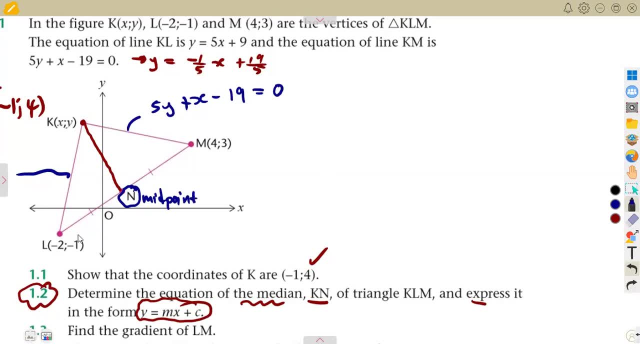 is a median line a line which divides this two equal paths if y a n here is a Even of for k what is the median loop 0, now if I have to determinate what is the median loop 0 at right it means that I have the median loop 0 therefore this is the median loop 0 plus 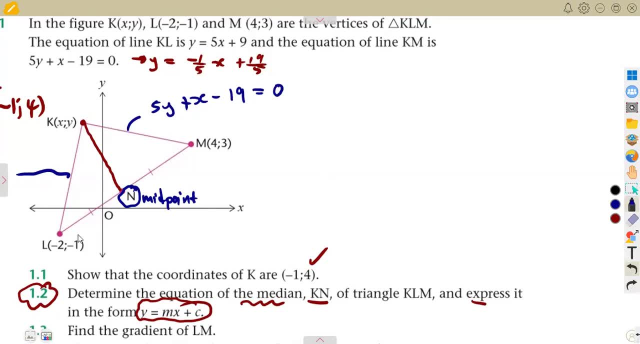 k open this I have the median loop 0 because you Jak is for the media so what if the median loop 0 and the median loop n were equal that could have been 0 that could be 0 because k and k had no end and it could have been 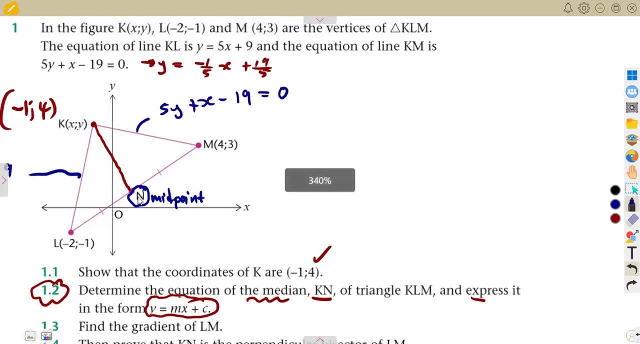 p k and g point k where k is the main point because it has Пом is a limit there that this 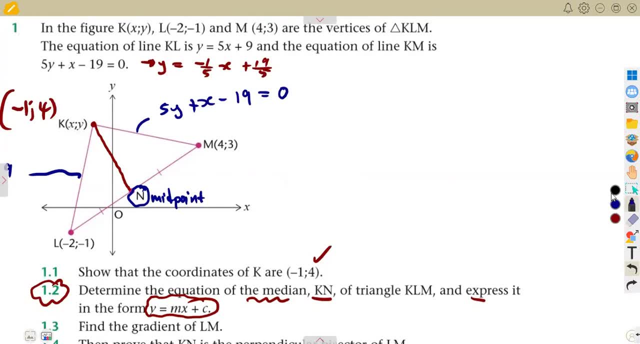 can've been marked in alpha but you jr佐 do not know the곱 do not know and for any other be fraternal or we are to be still as k for k in other behavior as a positive k 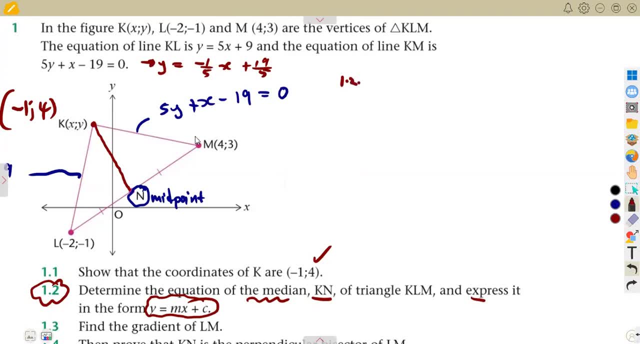 that's the case there all right 1.2 so like i said before uh n is the midpoint so to determine 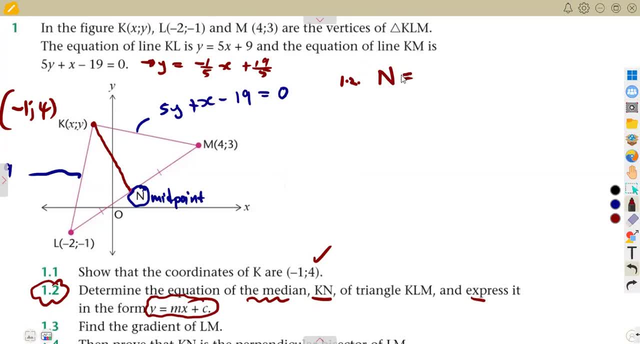 n which is the midpoint you are going to use the uh the midpoint concept okay so remember from our 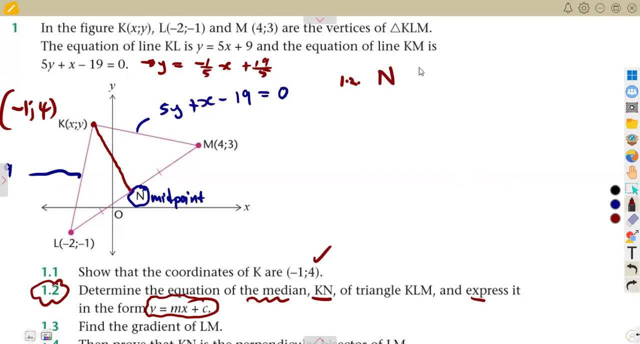 midpoint concept how do you determine this so you can write n is equal to or you can write any like 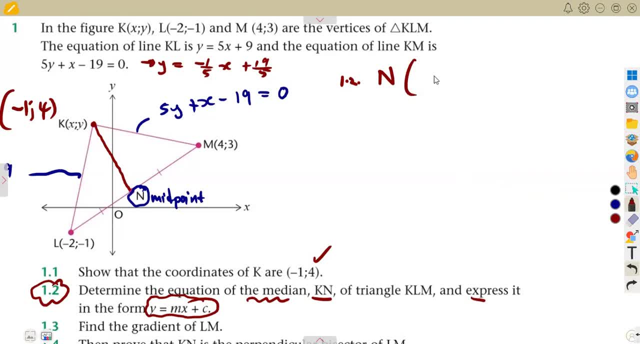 this representing a point n or you can write n is it guys no matter the way that you as long you 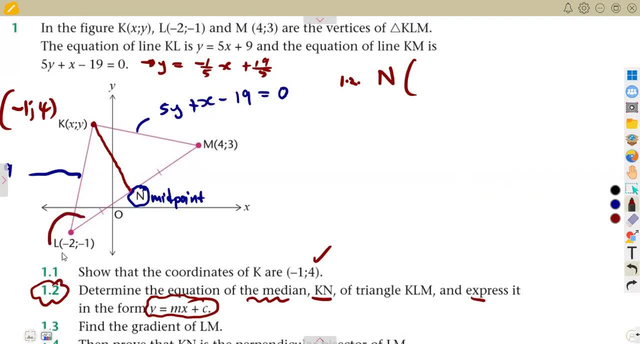 understand what you are doing there so n is the midpoint of what l m these are the two points 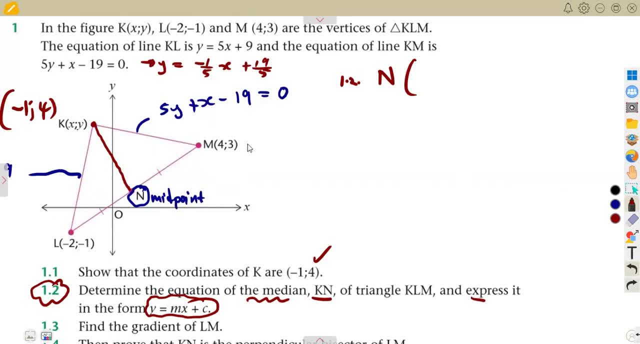 which lies on the line where n is so remember from the midpoint concept you said it's going to be x1 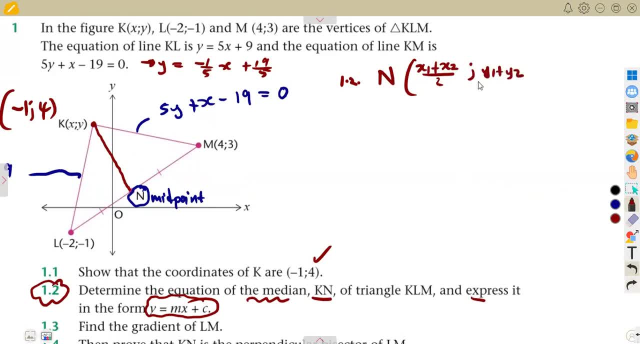 plus x2 uh into y1 plus y2 over 2 from the given points l and m we can use these two points as our 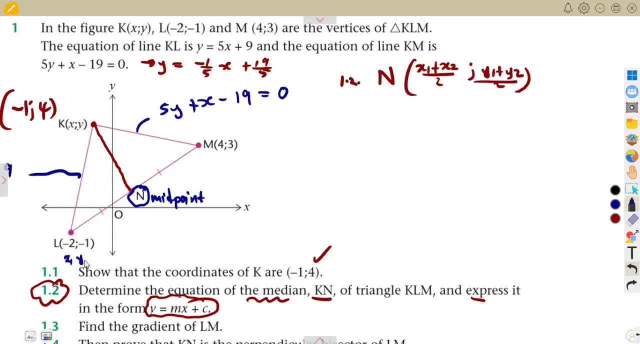 midpoints depending with the way that you're going to name your points you can have this as x1 y1 this is 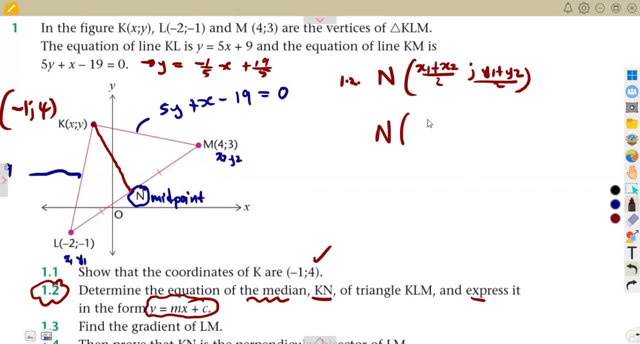 x2 y2 so that means n can be given as x1 that is minus 2 added to x2 on this point which is 4 over 2 then the y value which is minus 1 plus the y value on this point which is 3 everything over 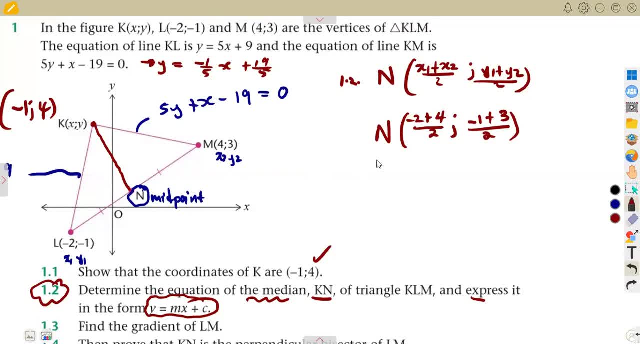 2 like i said before the way that you're going to name these points depends with you as long 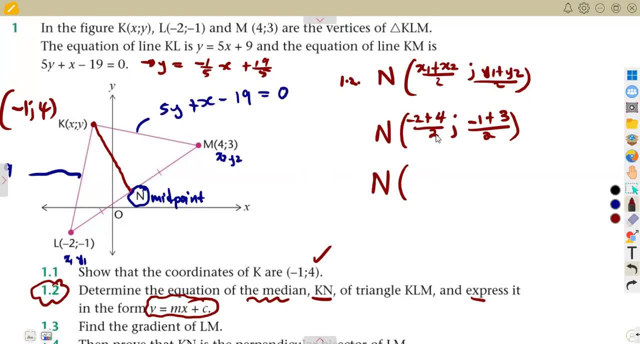 you understand that you are having the x values on their own the y values on their own so this was going to give us a one one on our calculator so that's the point n is there which is our mid 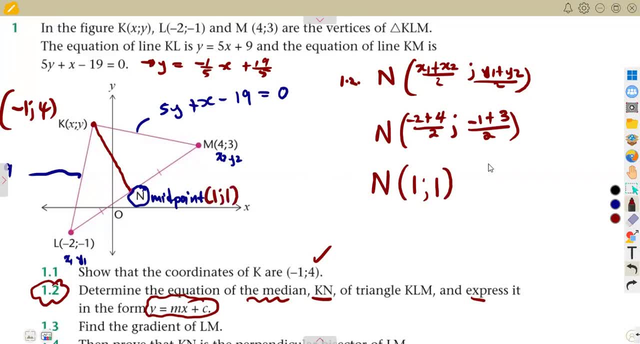 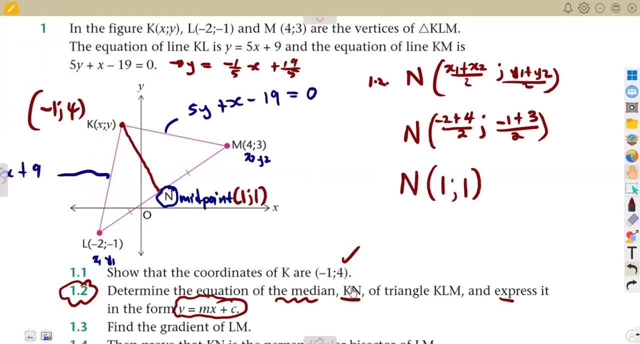 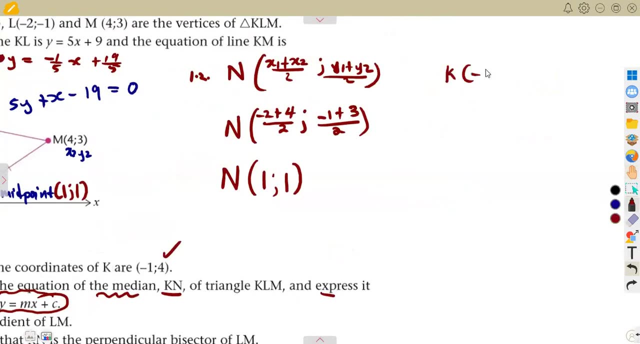 point so with n as the midpoint and with the k we can because we need to determine the equation of and we have the point k so given the point k which is minus 1 for the one that we're given there uh the one that we proved before we have the point k we have got 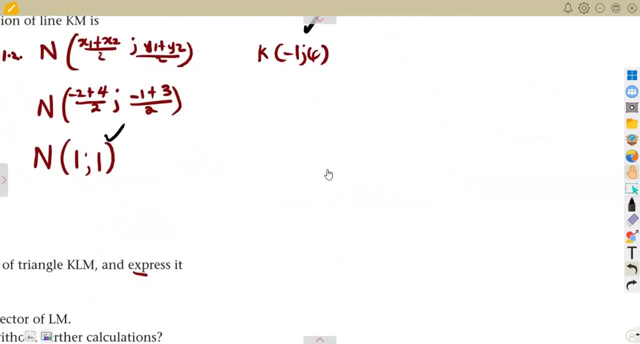 the point n we can determine the equation remember the question there is for us to determine what the 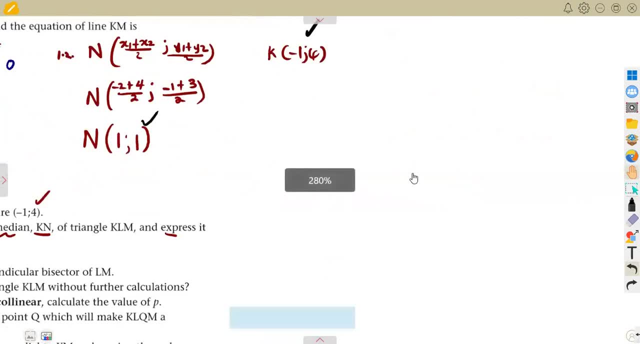 equation so how do you determine the equation given points that is the question when given 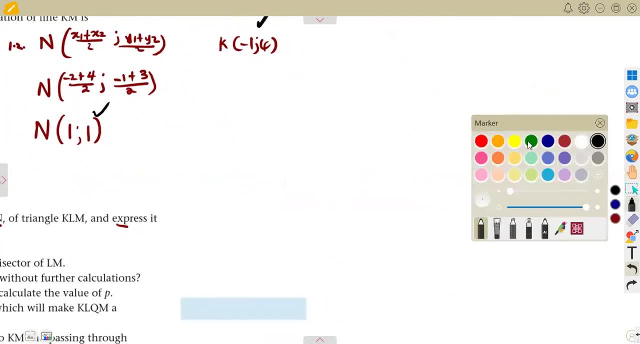 two points we can determine the equation remember the concept you are back again to that gradient concept you need the gradient first so the gradient of kn remember the change in y over the change in x 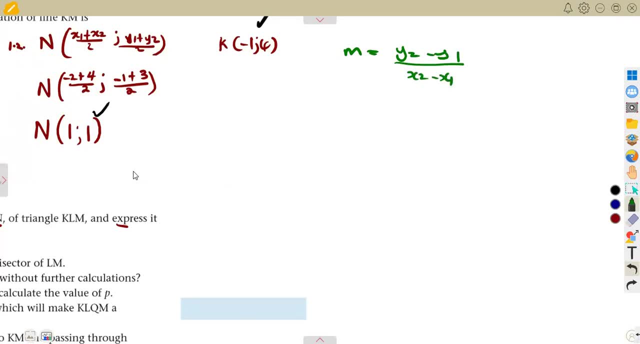 you so depending with the way that you are going to name your points maybe decide this to be your 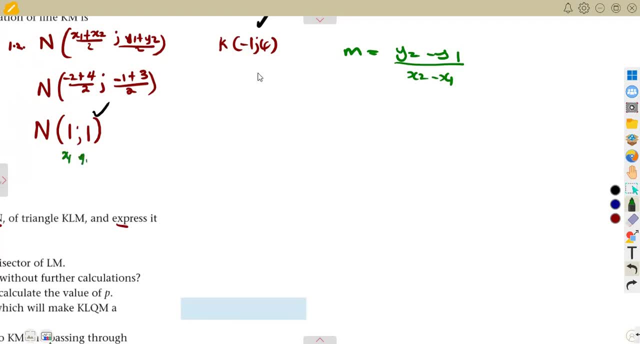 first point this to be your second point it's up to you x1 uh y1 x2 y2 it's up to you so this will be y2 which is 4 minus uh y1 which is 1 over x2 that's minus 1 minus x1 which is 1 so you are going to determine uh or here the gradient of the line that is uh 3 over minus 2 which is same as minus 3 over 2 with the method that you're going to choose i don't know 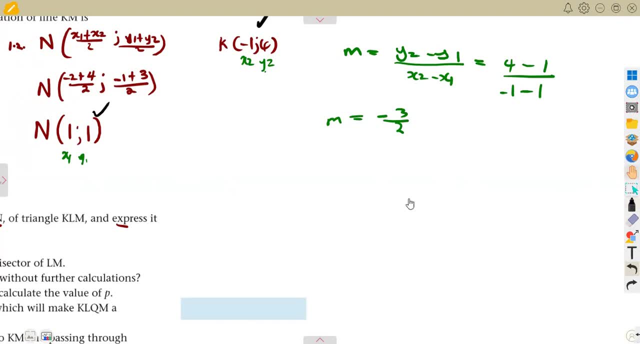 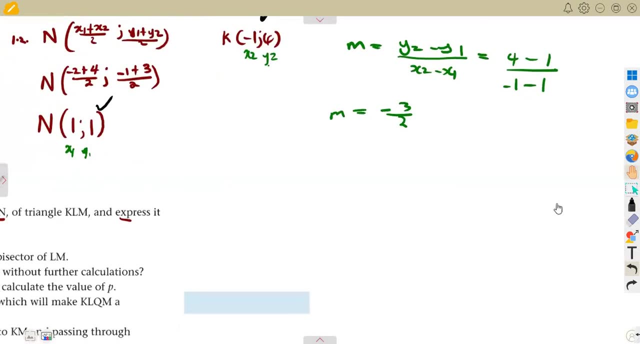 which method are you going to choose but you're going to have uh the answer in this format at the end so if you are already given this format i guess it's best that you also follow suit the format that you're given y is equal to m x plus c just substitute remember m is the gradient and we calculated that minus three over two x plus c which is the value to be calculated from any given point like i said before so i can choose to use the point n is the easier guys there is one 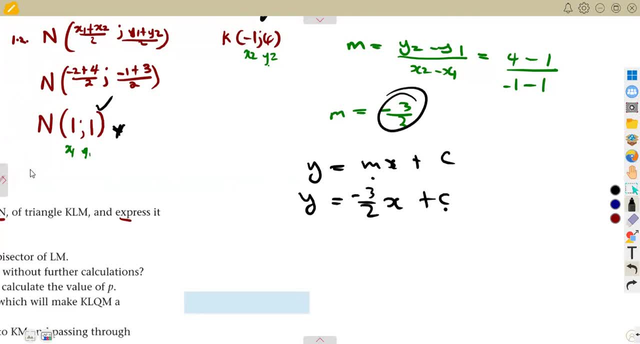 and one there's a negative there just choose what is easier for you all right so you can choose to work with the point n any part i'm not saying it's difficult but any part is uh just choose to work with what is easier for you so i'm going to use the point n which is one one that's x and y there so y is one when x is given as what when x is given as one you substitute into the equation minus three over two times one that's minus three over two we transpose e to this side it becomes a positive because it was negative the moment it crosses that's a positive there 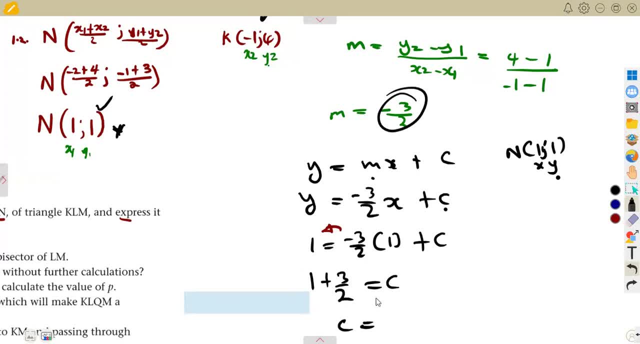 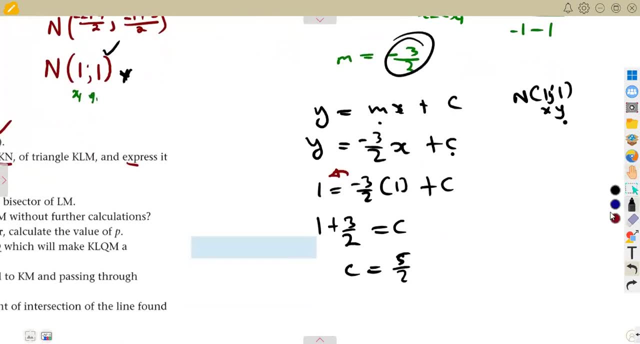 so c was going to be one plus three over two you're going to obtain five over two on your calculator so that's the value of c so having the value of c therefore our equation was going to be given as y 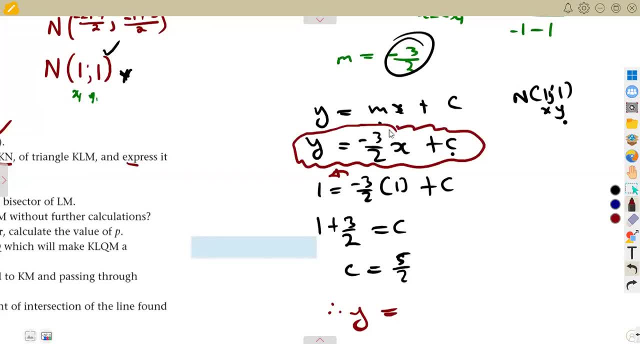 is equal to we substitute back to this uh part that you have already that is minus three over two x plus c which is five over two in exactly the format that you are given to express your answer as there is a format today you have a format that you're working with right right right right 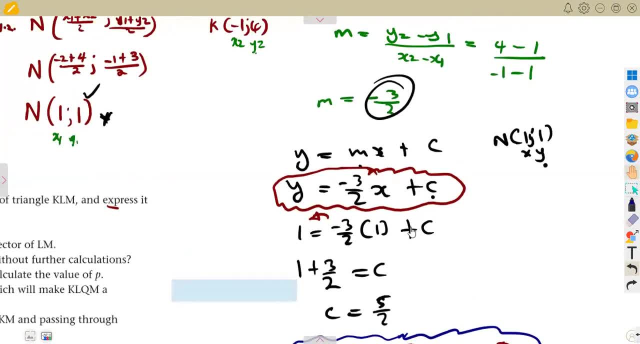 maintain that format you have to maintain the given format there so that was the equation 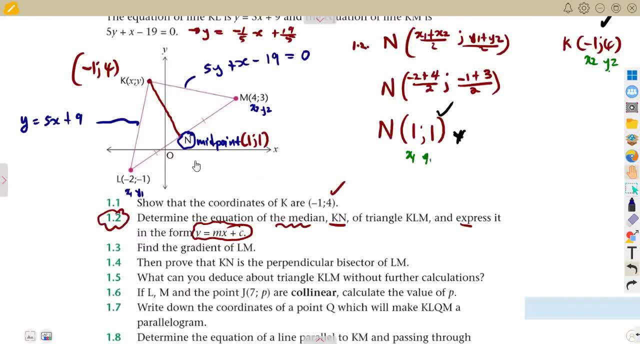 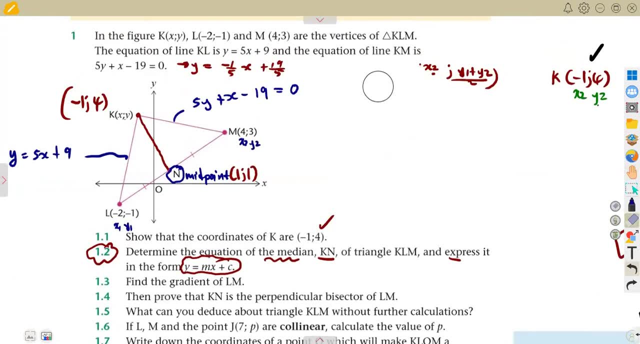 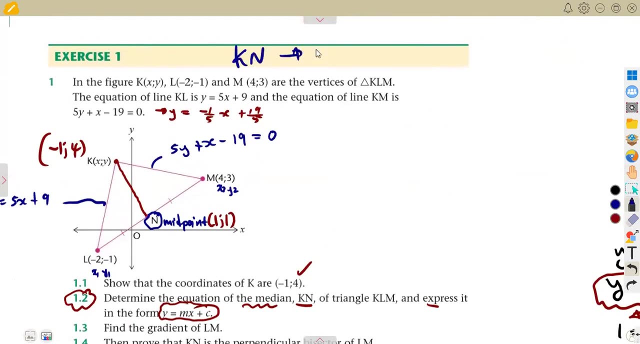 of the bisector which is this one uh so let us just write it aside we might need this like i said guys i just need to erase this so that we take advantage of this space that we have here so we calculated the equation of kn uh it's this equation was equal to y is equal to minus three over two x this is minus three over two x plus five over two remember uh still remember 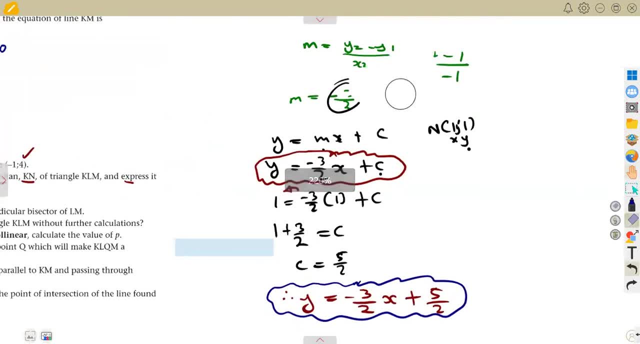 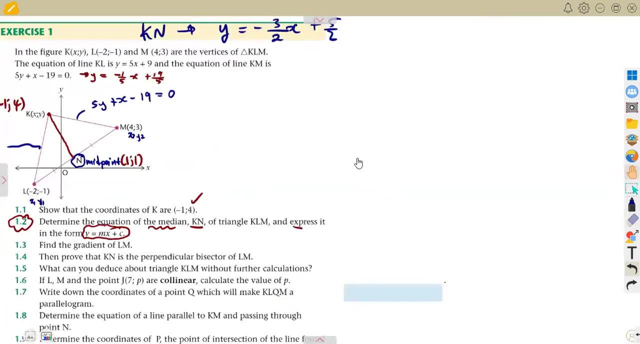 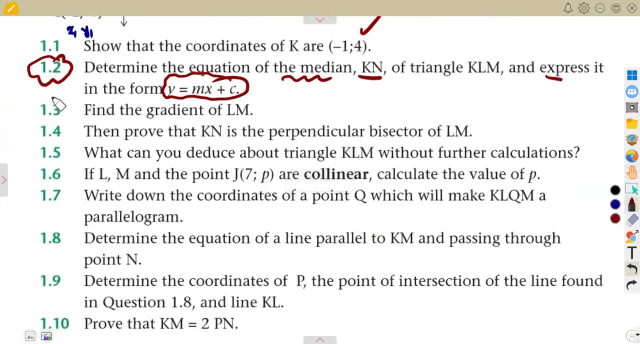 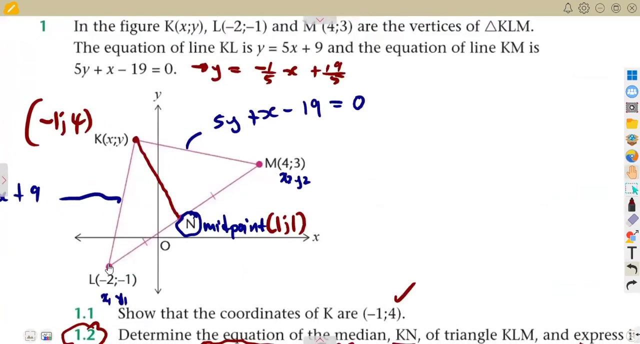 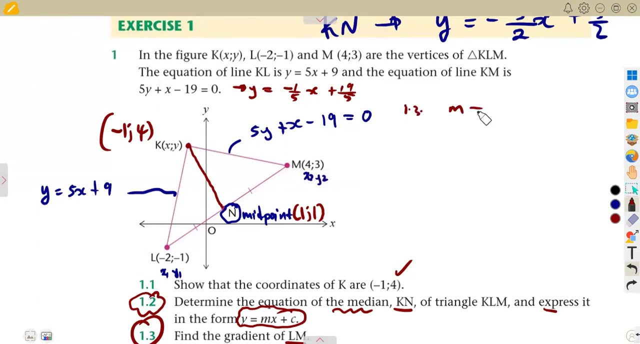 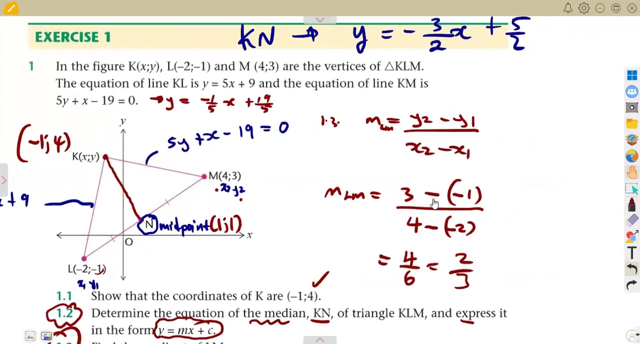 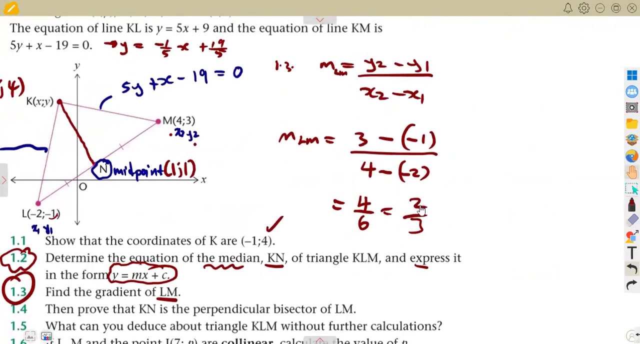 that that is what we got there my memory saves me very well all right so this is our equation uh we might need this we do not know so just so let us just read it aside find the gradient of l m on 1.3 so 1.3 is a direct question uh the gradient of l m are we having the point l are we having the point m the point l is there the point n is there so this is a very very direct question uh remember our gradient uh is just the change in y over the change in x all right so you can even write it as uh l m like l m so this is the gradient of l m which is y2 minus y1 already we stated this x1 before so it's going to be y2 which is 3 minus y1 there that is a minus 1 over x2 or x2 value that is for minus x1 which is minus 2 according to the way that i mentioned my points i indicated my points there the way that you mention the way that you indicate your points determines how you're going to substitute them on the formula uh that is idea there so that was going to be 4 over 6 which is simply two-thirds so you can just save your own on your calculator directly like that that is idea there so just remembering that your question is to calculate the equation uh you can now determine i mean uh the equation if you're given that consideration so this one it was just a gradient okay so we're done with that one all right so this one uh let 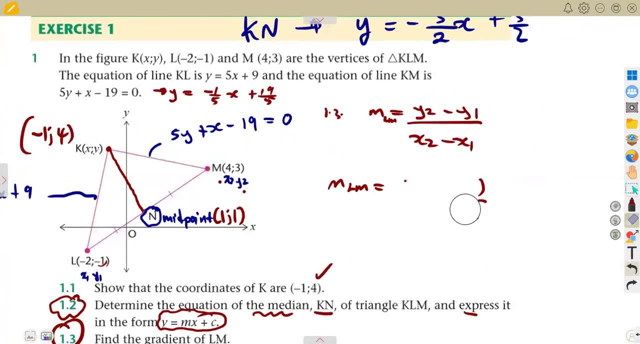 me just rewrite it here sorry for that so you see guys these softwares these softwares how they do react but anyways we just talk with time we'll be together 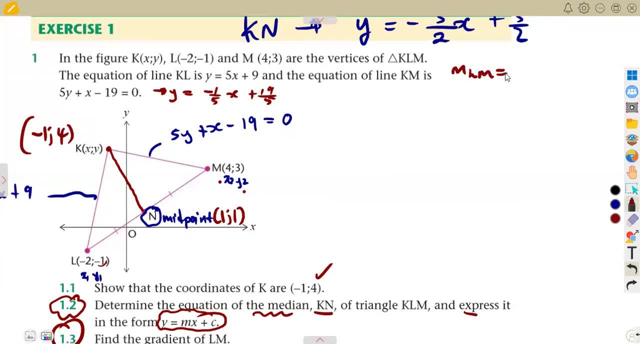 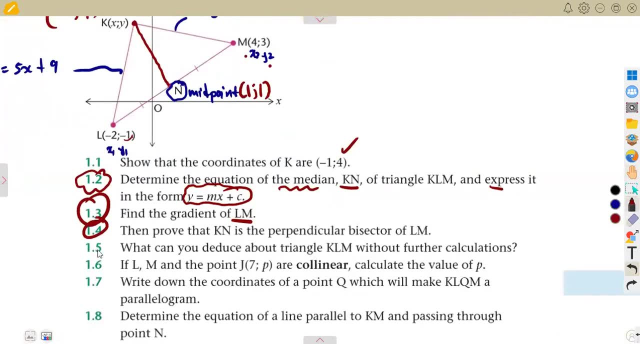 so the gradient of lm uh that is uh we go two over three so we are going to see maybe we might need that gradient later on 1.4 then it's a continuation meaning to say we're going to need 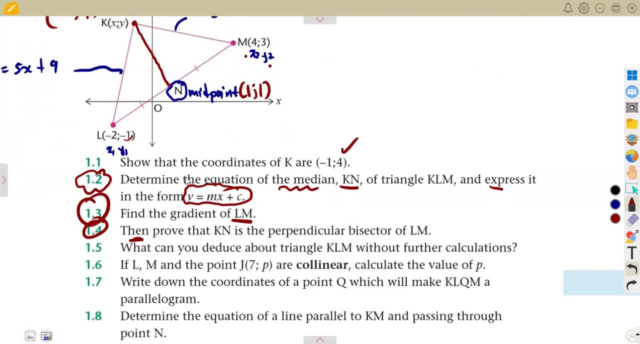 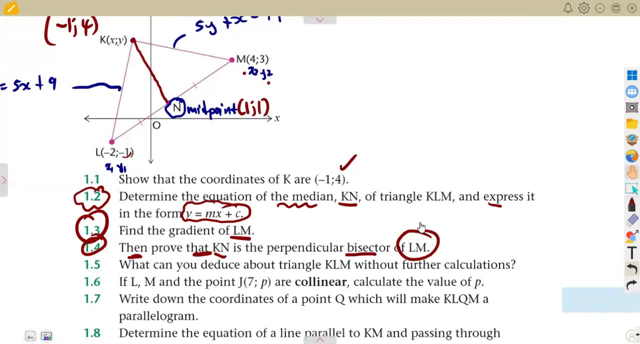 that one then it's a continuation from whatever that we did before so then prove that kn as the perpendicular bisector of lm all right before we did we talked about this remember kn this is our kn guys all right this 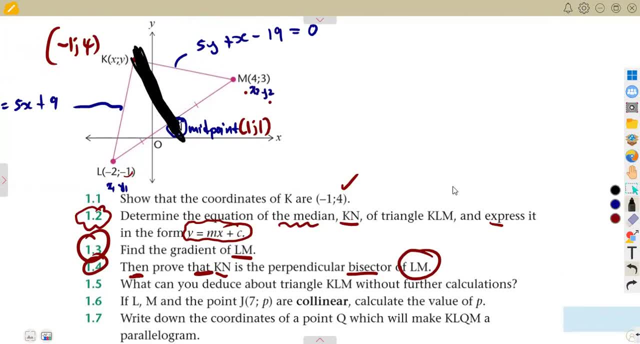 is our kn this one remember before we said n is the midpoint remember but here they are not only about to be a bisector to bisect guys it means to divide into two equal parts that is to divide that is to bisect to divide into two equal parts but this is not about just bisecting it is a perpendicular what is it there about being perpendicular being perpendicular means they have to meet at 90 degrees so it's no longer about just being a bisector there understand your 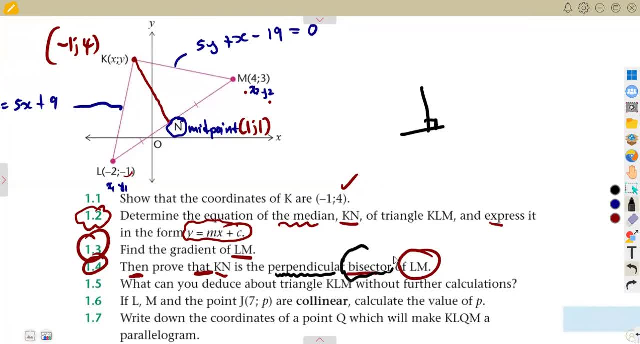 question so the midpoint or the bisector part we are not focusing on it no we're not focusing on that because already we're told that this is the median kn and we we say this is the midpoint of midpoint so now they want us to prove that this line kn is at 90 degrees that is what they want 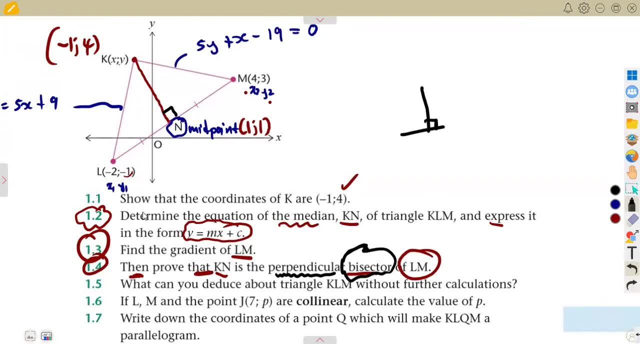 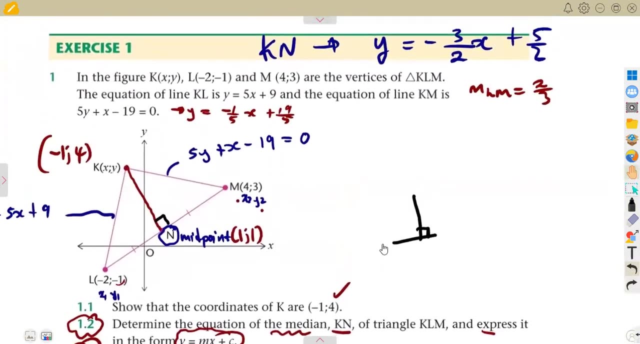 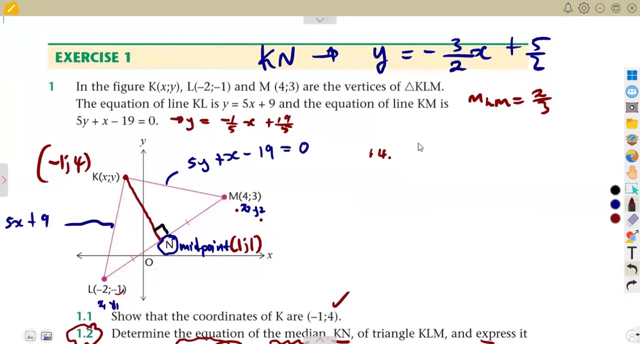 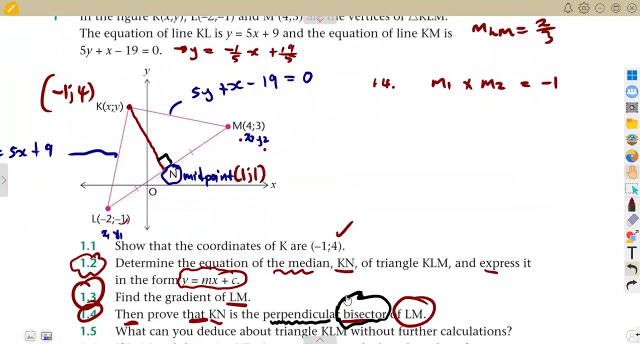 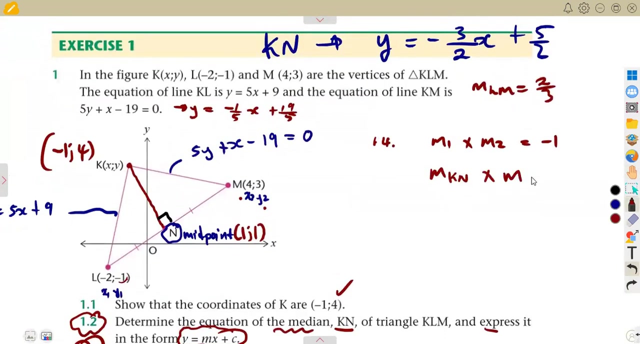 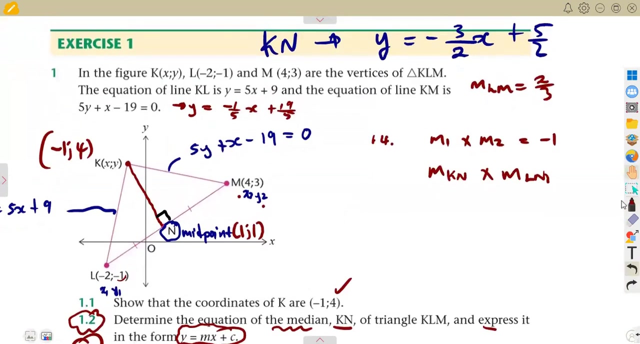 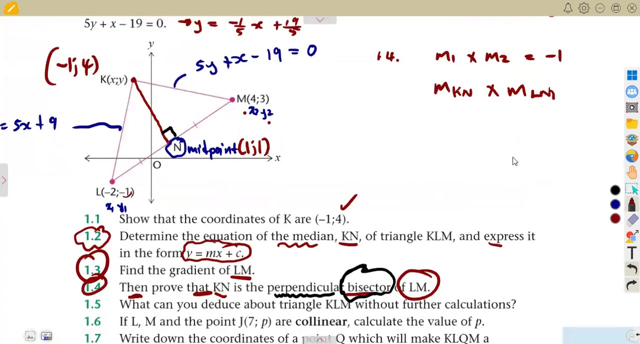 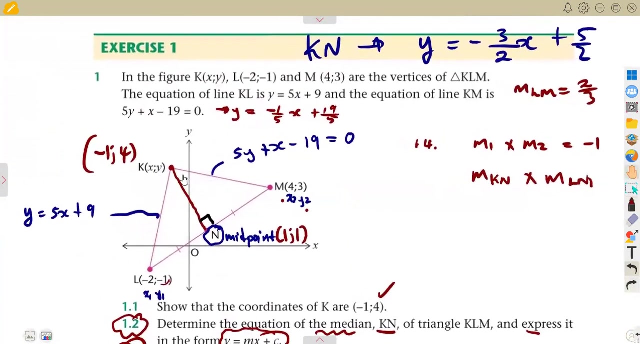 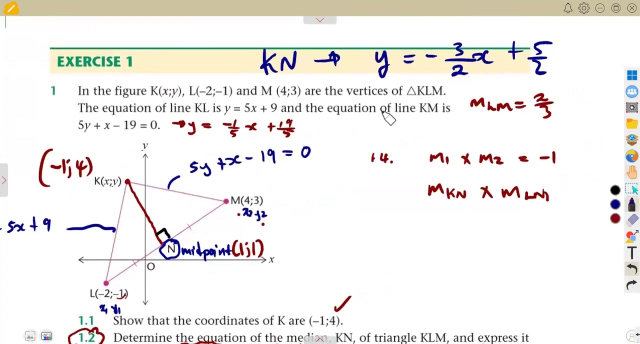 you to prove because the bisector concept is done it's done the bisector concept is the one that we had before the midpoint concept so we need the perpendicular part so what is going to be it now about being perpendicular all right that's 1.4 so for these two lines to be perpendicular remember what i said uh on the introduction that two lines are supposed to be perpendicular if the gradient of the two lines is equals to negative one that means what we need to prove is this case is that line kn kn and lm so meaning to say the gradient of kn times the gradient of ln which is lm that that line that you're given is lm should be equal to negative one this is what we need to prove if we can prove this then we are done all right so let's see uh we have the gradient of kn the gradient of kn are we having this where is our kn this is k to n this one remember when we calculated um this equation here of kn we had the gradient it's only that i erased but for this one we can even take it here kn this was our gradient the one that we calculated remember it was minus three over two so meaning to say minus three over two times the gradient of lm the gradient of lm that is two over three all right so if you had to use this on your calculator if you had to use your calculator that was going to give you a negative one so as we can see we are obtaining a negative one 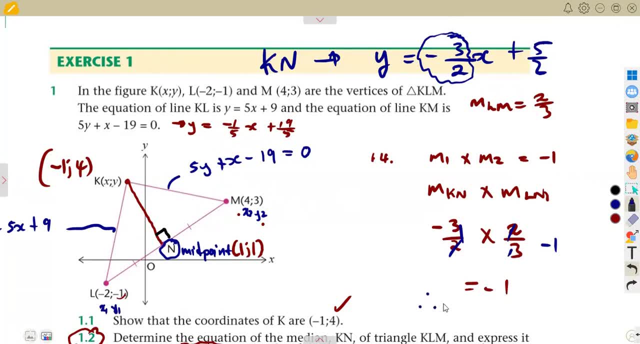 to obtain a negative one thus therefore 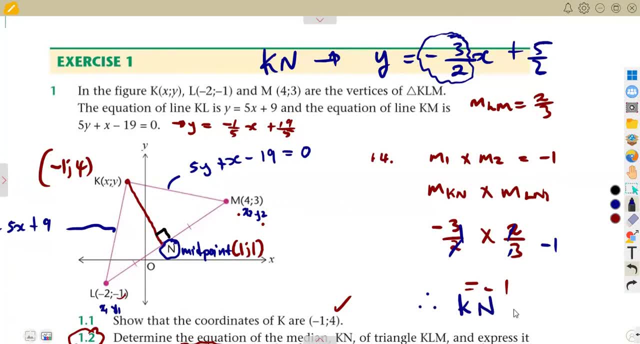 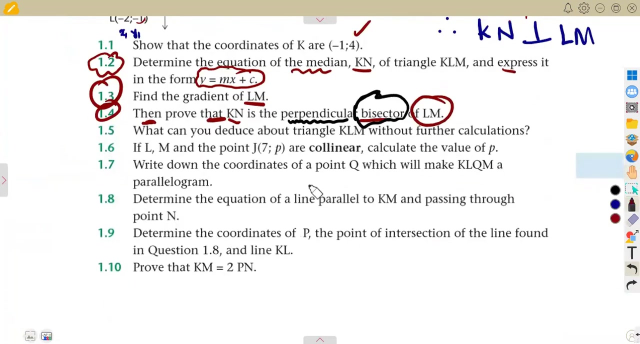 these two lines are perpendicular so therefore kn is perpendicular to lm all right that is it that is to say kn is not just a bisector but it is a perpendicular bisector it bisects this line at 90 degrees that is being perpendicular it bisects at 90 degrees that is the idea there all right 1.5 what can you deduce about triangle k lm without further 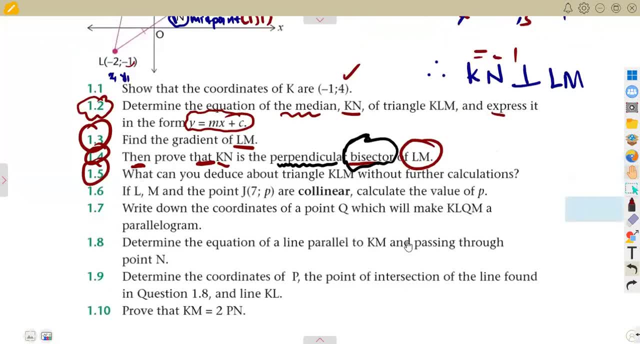 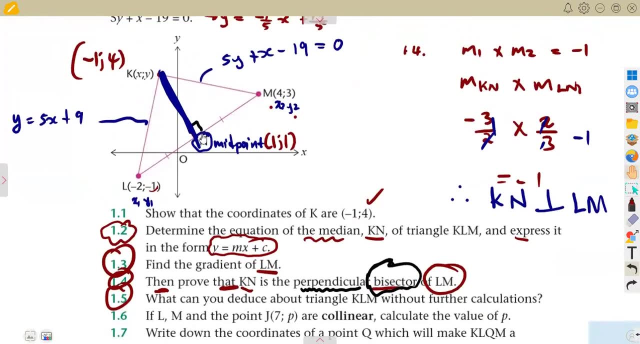 calculations what can we say about triangle k lm this is our triangle k lm what can we say all right we saw that this is at perpendicular it's at 90 degrees bisecting this line into two equal parts there is nothing but it is an isosceles triangle remember the isosceles triangle concept uh this is the idea them the isosceles triangle 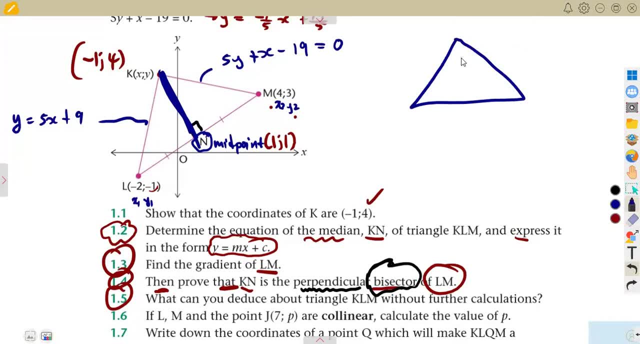 concept uh i'm not saying it it can be also an equilateral triangle so what is important is that if a line is drawn from one point which is the vertex bisecting this other line that is at perpendicular at 90 degrees bisecting this line into two equal parts it follows that these two lines are equal in length so if this line this line and also this line are all equal it becomes an equilateral triangle but if it is only these two lines which are equal but they are not equal 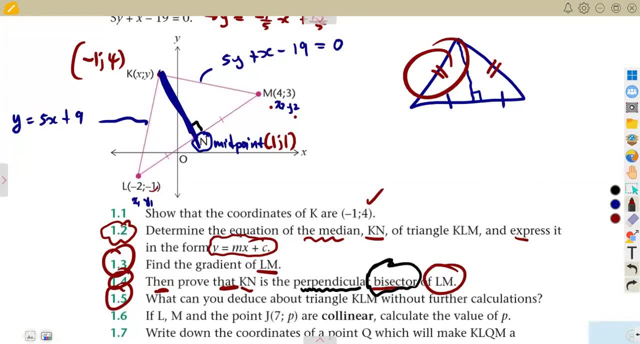 to this line then it becomes an isosceles triangle so we can't say it's an isosceles 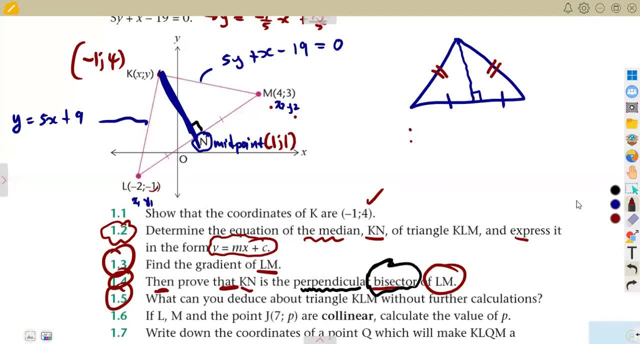 triangle or we can't say it's an equilateral triangle but we can deduce that uh that is the idea there so 1.5 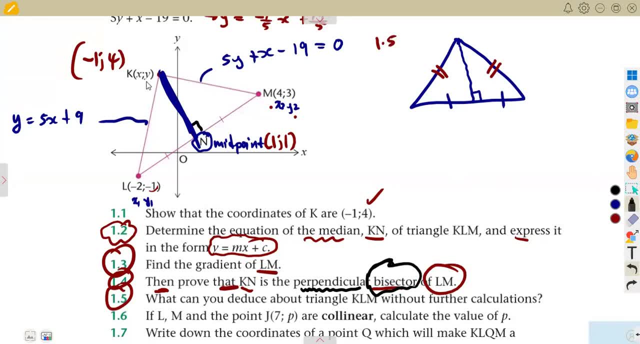 we can deduce that this is what we have uh from k to l this line is equal to k to m all right so we can deduce that k l is equal to k m that is the idea there 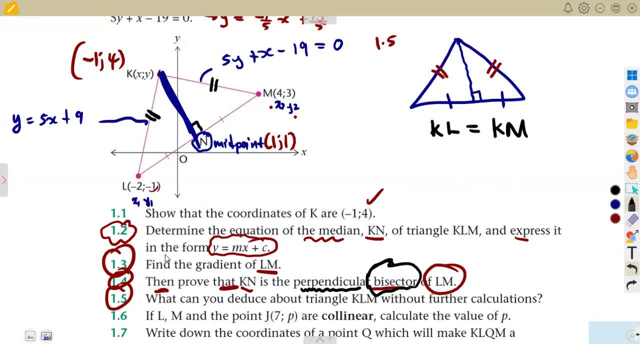 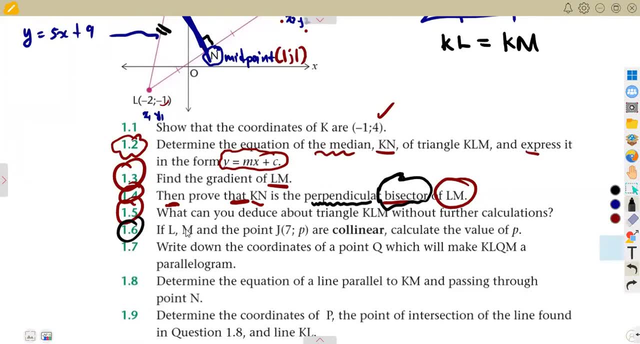 so be careful on your presentation that is what we have uh 1.6 if l m and the point j given as 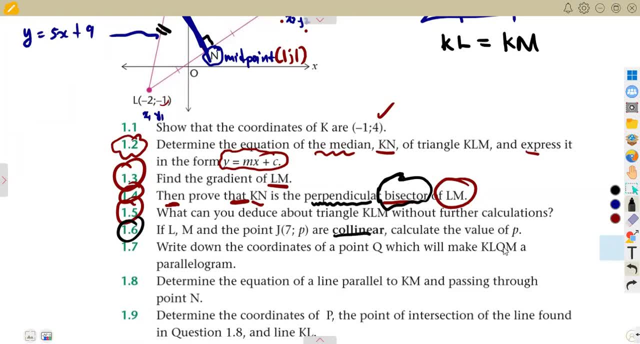 7p are collinear remember i talked about the collinear points on the introduction calculate the value of p if these points are collinear all right let us have it here 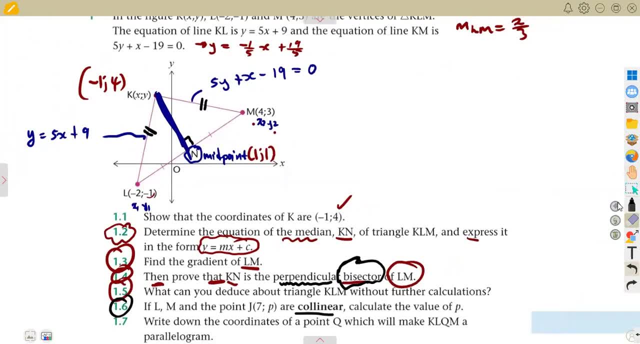 i hope you understand me on this that's 1.6 so we are given the point l the point m and the point j which we do not know of that is the value of p so we are given the point j 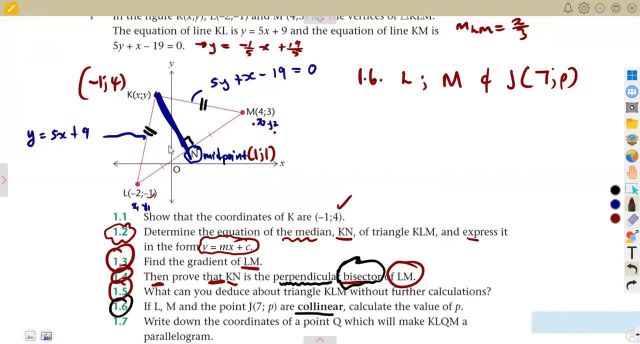 that we are not even having on the diagram we do not have that but l and m are the points on the 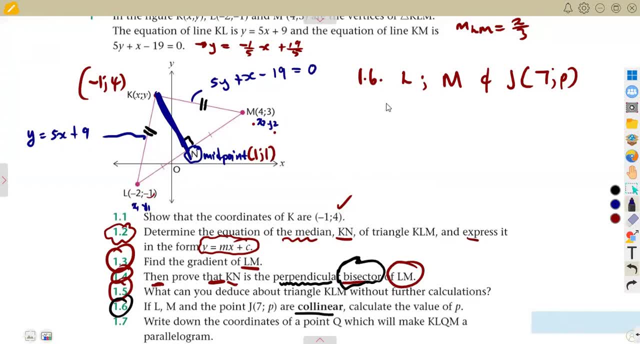 diagram the point l is given on the diagram this is minus 2 uh minus 1 that's our point l 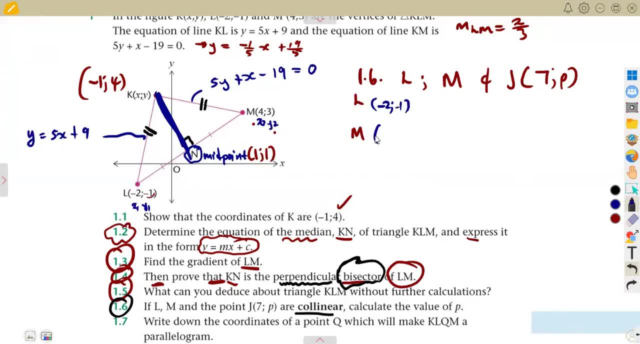 and also the point m is there on our diagram which is for 3 so what is it that we can take 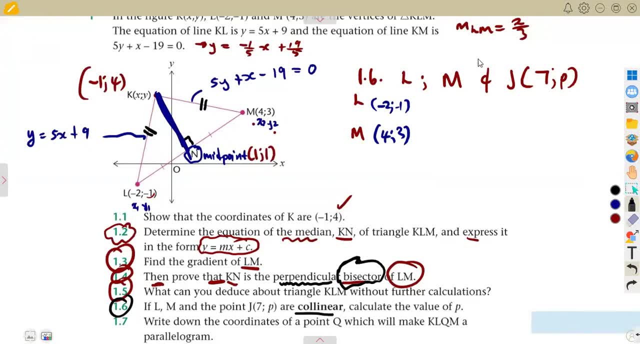 about the collinear concept if points are referred to as collinear 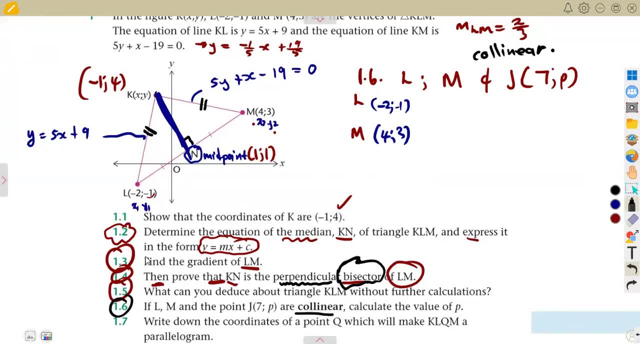 it means that they lie on the same line they have got the same gradient if i'm to consider any 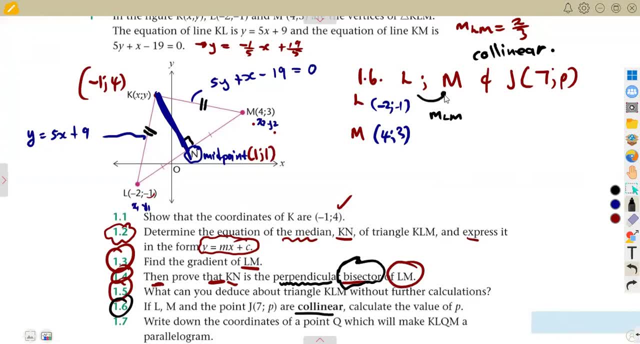 point the gradient of l m these two points must be equal to the gradient of m j uh in that case it must be equal to the gradient of m j all right the gradient of m to j it is also supposed to be equal to the gradient of lj 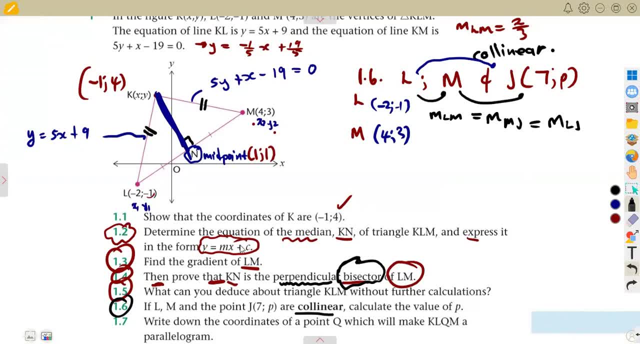 j whatever way that you are going to as long you are taking two points so taking that as an advantage because we have the gradient of l m the gradient of l m here we calculated it before it was two-thirds so we have the gradient of m l m before which is two over three so what we need 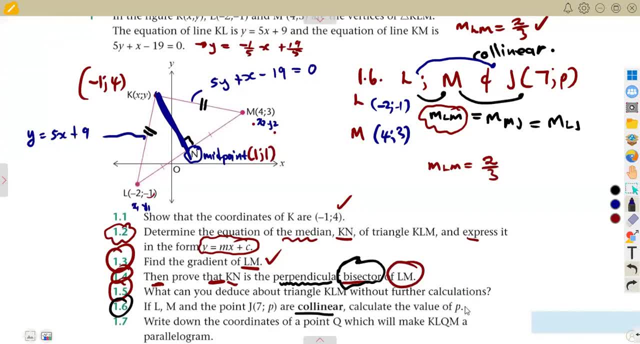 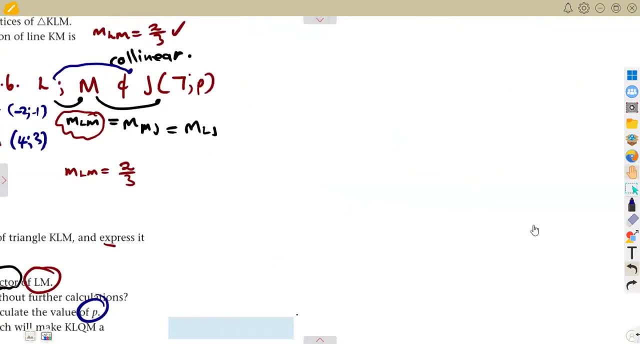 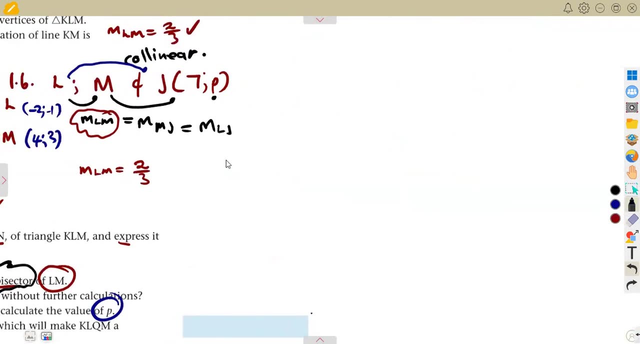 there is in order for us to have the value of p this one we are going to use the point j which has got p that's where p is p is on the point j so you're going to take any part that you want is it m and j is it l and j it's up to you so in this case i'm going to use m and j to find what the gradient so i'm going to determine the gradient of m j 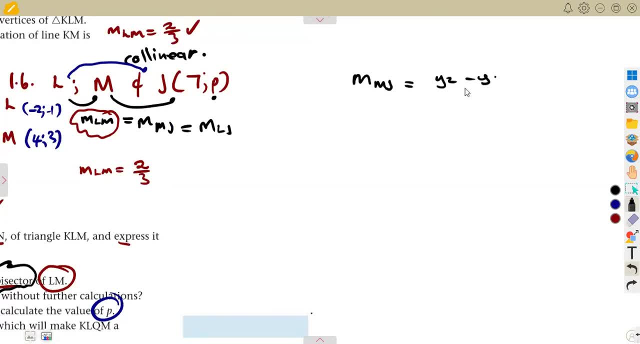 all right remember the gradient change in y over the change in x that is our gradient concept so using m j that means i'm gonna refer to this m as x1 y1 this as x2 y2 is up to you how you're going to name it so y2 is p that is going to be p minus y1 which is three everything over x2 which is seven minus x1 which is four so 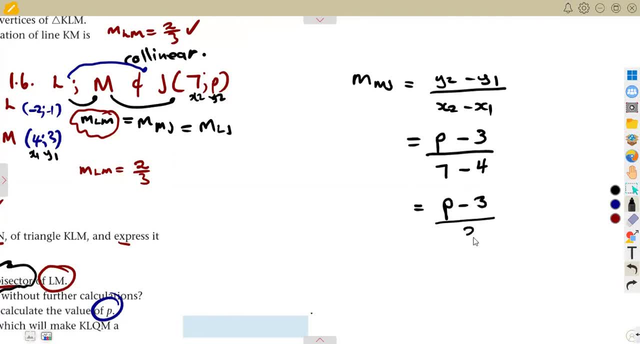 that is our gradient concept so using m j that means i'm going to refer to this m as x1 y1 this is going to be p minus three everything over three so this is the gradient of m j so knowing that 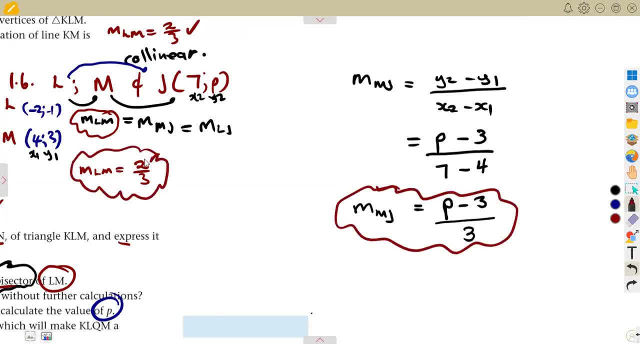 these points are co-linear they are on the same line they have got the same gradient i can equate these two gradients together because i understand that they are equal these two 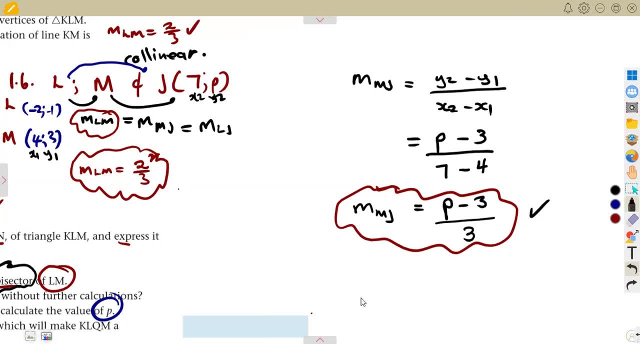 so it follows that this gradient of p minus three over three is equal to the gradient that we numerically have in of lm that's a numerical value this one is in terms of p so 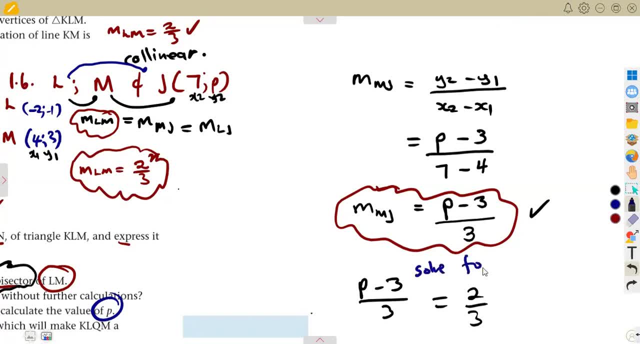 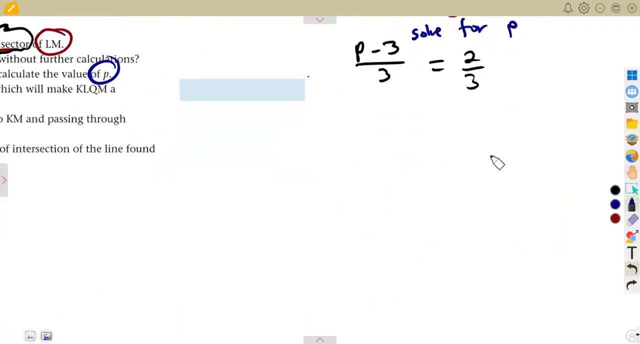 from this you can solve for p that's an equation now you have an equation so how are you going to solve for p it's either you're going to cross multiply it's up to you but if you can check here 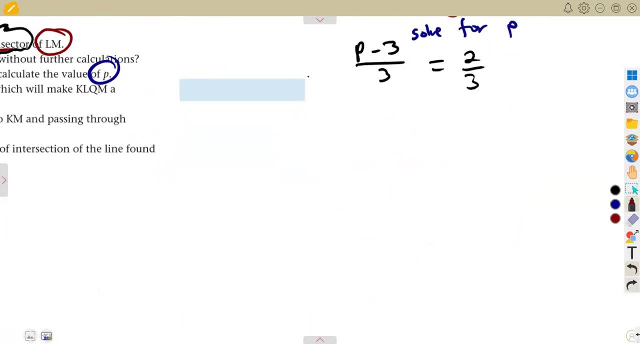 the denominators are the same so if they are the same you can take it as an advantage guys this concept here that i want you to understand 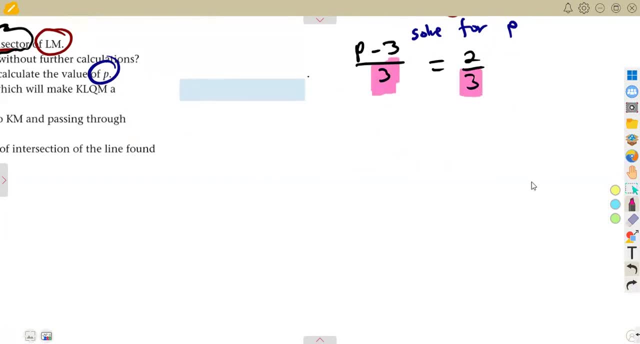 now we are at a higher level uh we could have talked about this in grade 11 but now you i mean 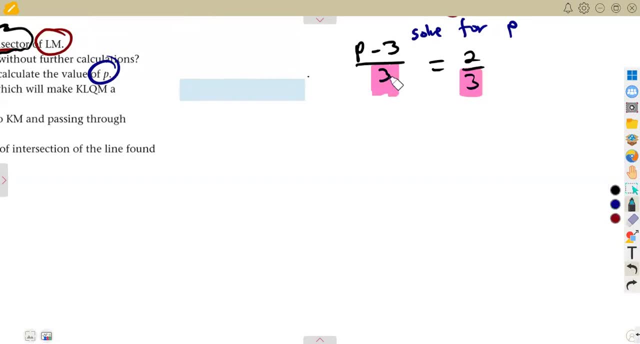 in grade 10 but now you can understand me guys it follows that if the denominators are the same like this you're solving an equation just equate the numerators so it means therefore p minus three 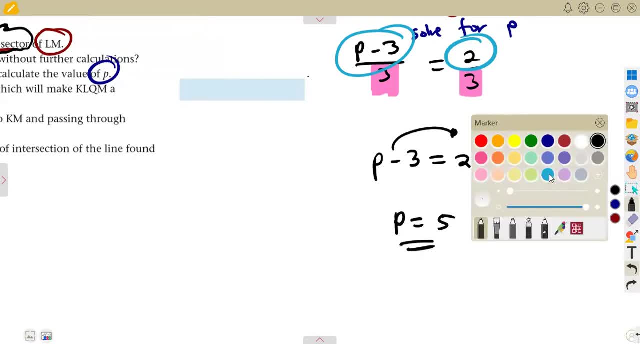 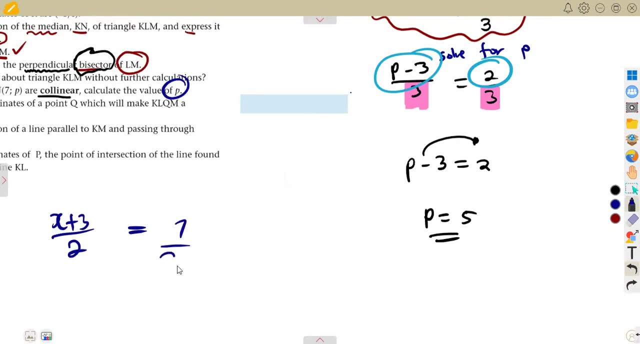 will be two plus three which is five so what am i trying to say if i am given an equation like this this is x plus three everything over two and we are given this as seven over two instead of you 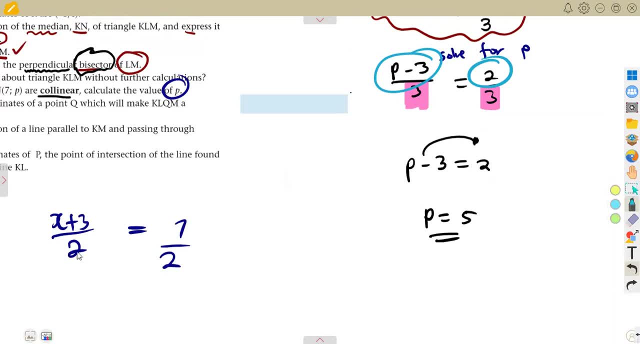 to cross multiply yes you can do that but instead of you doing that because the denominators are the same you can take advantage whenever it is like this you can take advantage of this you just equate the numerators so it follows that 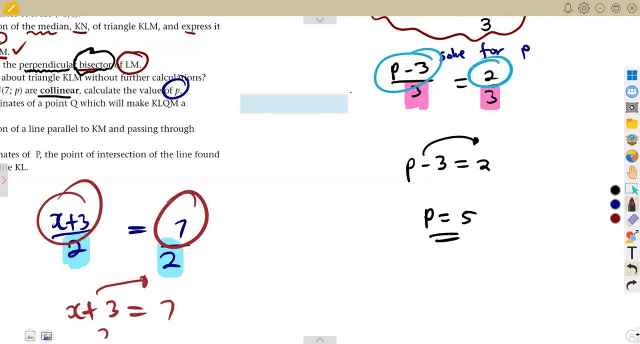 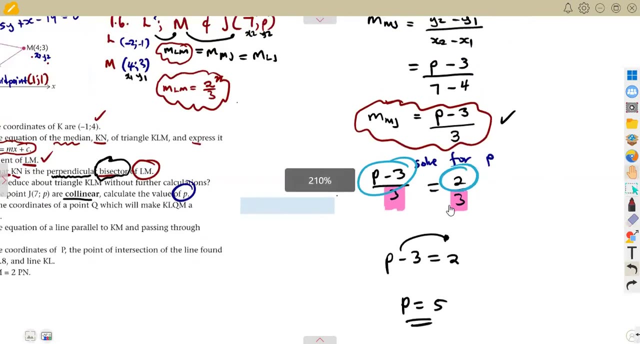 x plus three will be equal to seven transpose this x is gonna be seven minus three which is a four that's the idea there so meaning to say we can solve any equation as long the denominators are the same so we have got ways guys so i want you to do the cross multiplication and prove if we 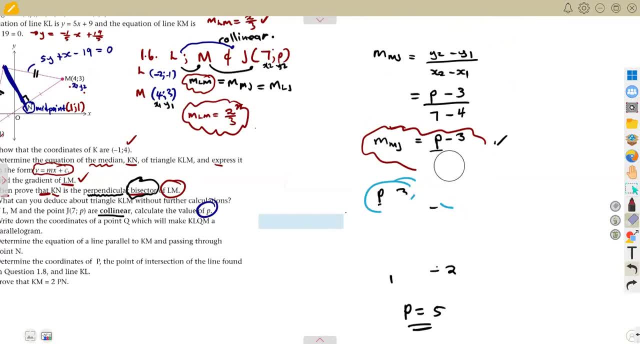 are in the same direction so that is the value of p uh let us remember this in case we are going to need this let us just remember our value all right let us consider 1.7 the coordinates of the point 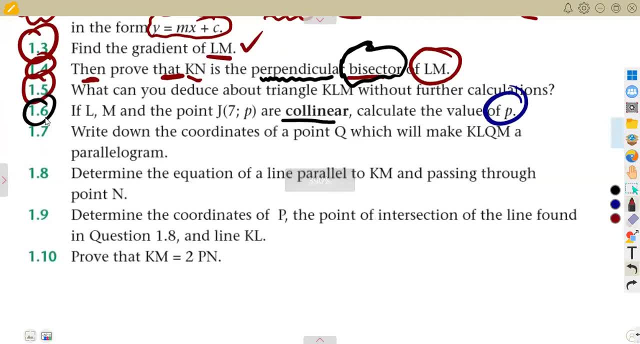 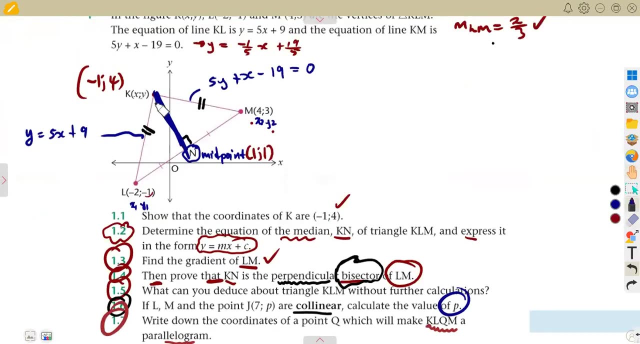 q which is going to make this whole part of k l q m a parallelogram all right the coordinates of q let's check where are we having these points k l whatever that we have there so this is where we have our points kel i mean k here so whenever you are getting 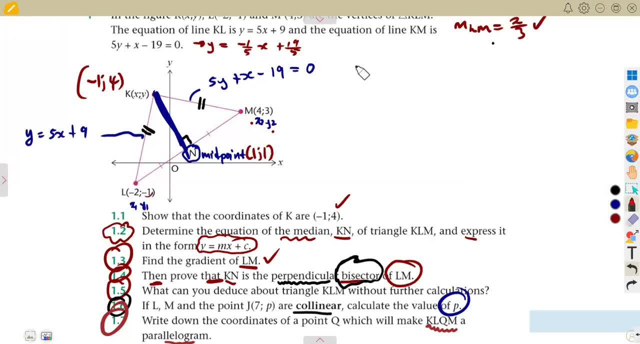 given this you are supposed to follow suit the order that you are given the order that you are given is important you need the coordinates of q you do not know about this point q so you can just 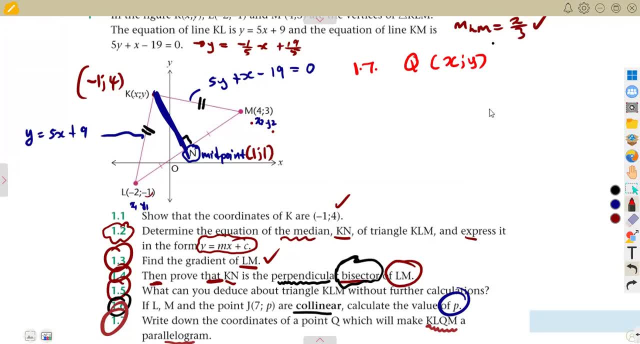 call it x y but it is supposed to form a parallelogram which is referred to as k l q to m so i am supposed to follow the order from k to l that means there is a point q somewhere there to point m so that i'm gonna form a parallelogram something like this where these two sides are parallel to each other and also equal these two sides parallel and also equal and it also follows that if this is my point q here which is referred to as x y the midpoint which is our n is going to be common remember n is the midpoint of l m l m is going to be a diagonal we have a diagonal there remember the concept about a parallelogram back now to the properties of your shapes from your grade 10 from our grade 10 we said these diagonals of a parallelogram they bisect each other at a certain point they do bisect each other meaning this point n is the common midpoint so n is the common midpoint it is going to be the common midpoint of the diagonals of the given diagonals of the diagonal so what am i trying to say if n is the midpoint of the given diagonals and we have that point n remember n is given as one one it means we can use the midpoint concept to calculate the point q because this k to q it is a line which passes through the point and it's a diagonal 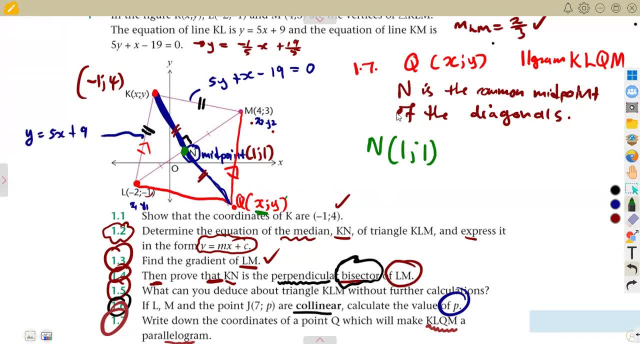 and it passes through the end because the common midpoint for the diagonals so meaning to say it is also the midpoint of what it is the midpoint 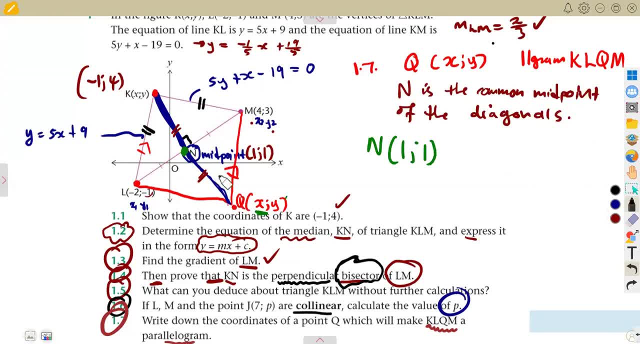 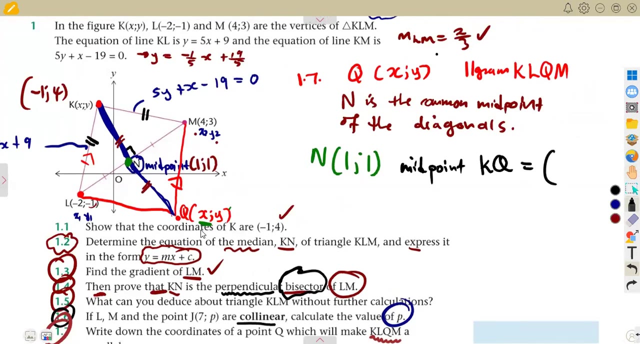 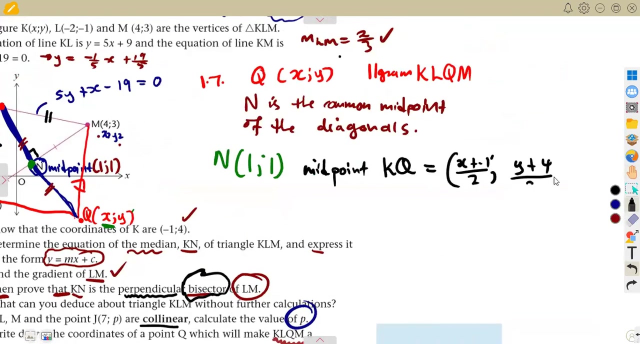 k to q why am i consider k to q because that is where i am supposed to calculate the value of x and y on point q so using that let's say we have got the midpoint uh of k q what is going to be the midpoint of kq the midpoint of kq remember the formula x1 plus y1 so it's going to be the x value to the x value on the other side so let's say we have got x1 plus y1 so it's going to be x plus minus 1 over 2 the y value at this point uh q which is y the y value at this point which is 4 so this is y plus 4 over 2 this is what you were supposed to have y plus 4 over 2 as your 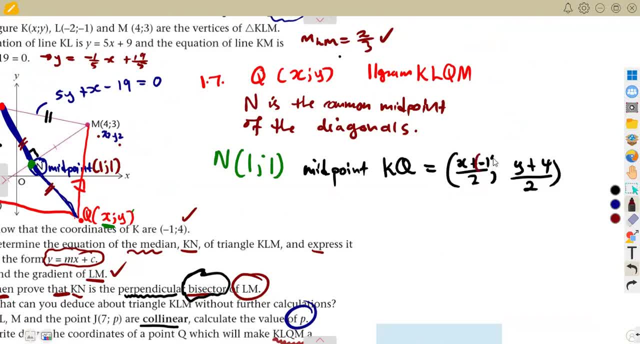 midpoint uh in terms of what in terms of x and y the ones that you're given the same midpoint is the same as this one because we say it is the common midpoint so if it is the common midpoint and i can write the same midpoint in terms of x and y like this 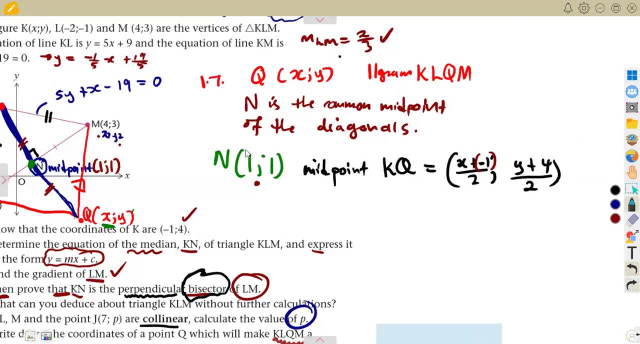 and i want to calculate the value of x and the value of y i can simply equate because this is the x value the y value the x value the y value so it follows that the x value at the midpoint must be the same there is no way that 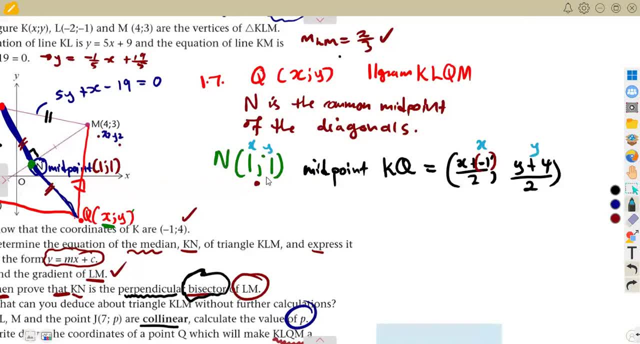 a n is the midpoint which is 1 1 then we calculate the midpoint of kq which is a diagonal because we are saying it is the common midpoint of the diagonal 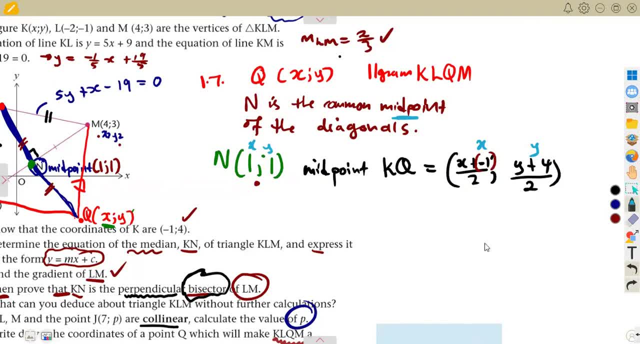 we calculate the midpoint of this diagonal we get something like 1 3 it's impossible why is this is 1 1 we are supposed to have the same value the same if we calculate the midpoint of this it is supposed to give us 1 1 so it means this is equal to 1 this is equal to 1 that is what it simply means there's no way we can have different uh values of x at the midpoint while at least we said it is the common midpoint of x and y so this is the common midpoint of x and y it is the same midpoint 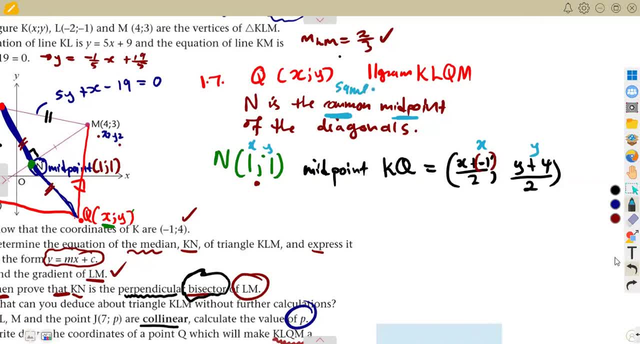 it can be so it means that this one for x all right so considering for x this one must be equal 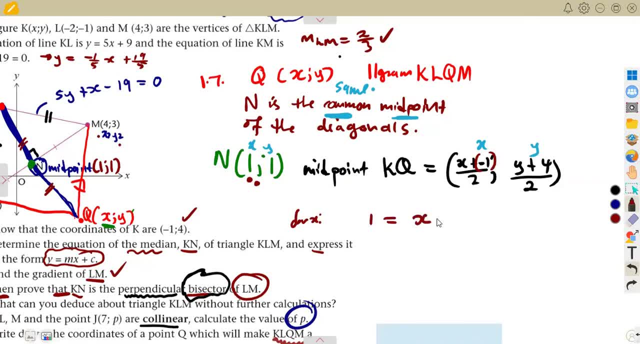 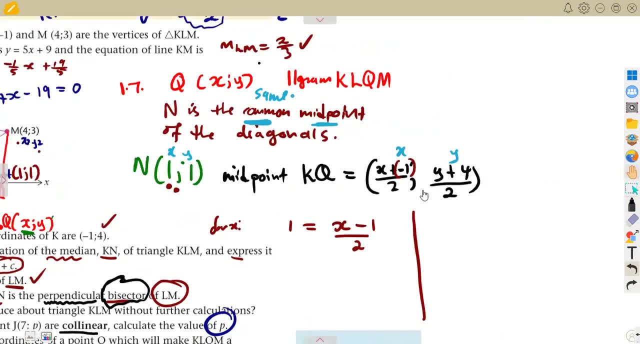 to the part of x here which is x plus and minus that is a minus over 2 we have formed an equation for x the same thing for y if we are to do this we are going to equate and form an equation there so for y we are going to take 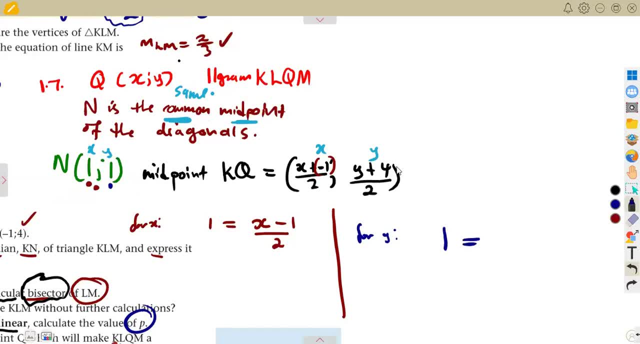 the y value at the common midpoint to the expression or to the presentation of the y value of the same midpoint in terms of what in terms of y so with this we can solve the given equations 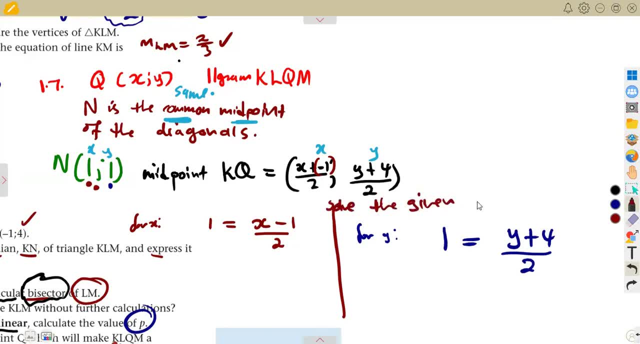 solve the given equations so in this case we are going to solve our equations uh this is 1 over 1 so remember i said you can make the denominators to be the same but if you do not understand the 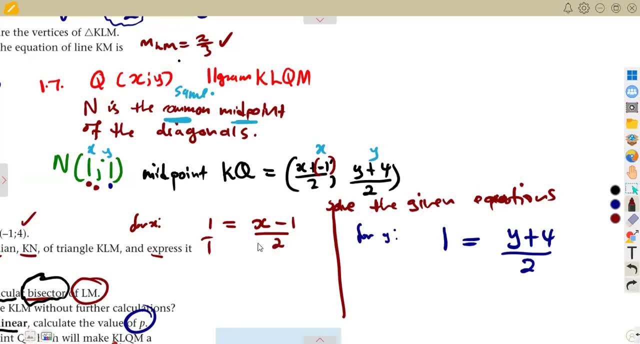 question that on this case they are different so just proceed with your cross multiplication or you can write this as 2 over 2 then you equate the numerators or you can just cross multiply 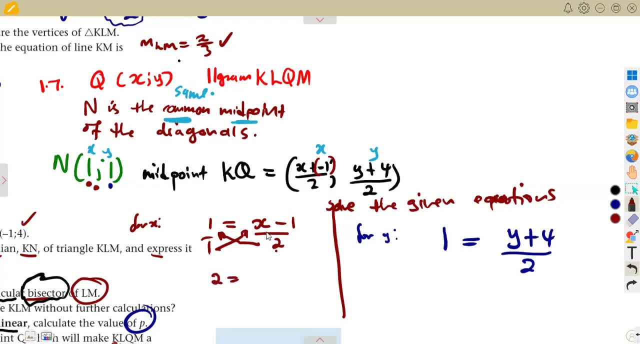 2 times 1 that is 2 is equal to 1 times anything it remains as it is transpose the negative 1 it 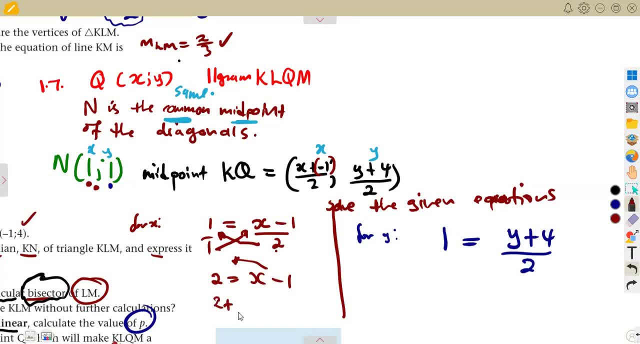 becomes a positive so 2 plus 1 uh is equal to x so that's x is equal to x is equal to 3 so like i was saying you could have written this 1 over 1 it is the same thing but you can write it as 2 over 1 and you can write it as 2 over 1 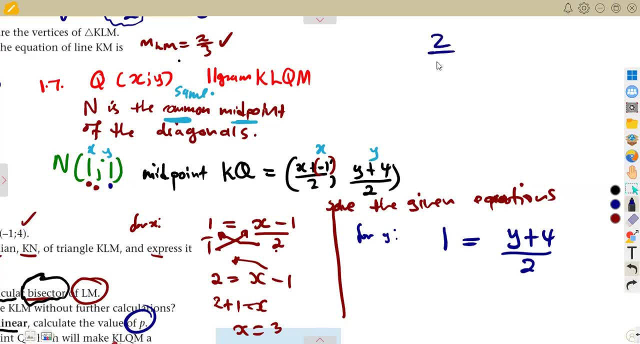 it is the same as 2 over 2 also to get a 1 we just need a 1 so 2 over 2 y 2 because we want the 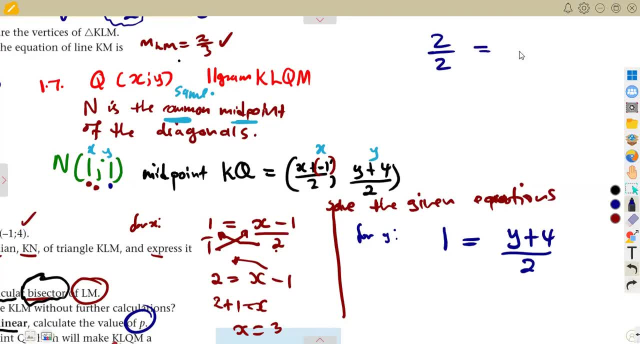 denominators to be the same so 2 over 2 is equal to x minus 1 over 2 by having this i simply 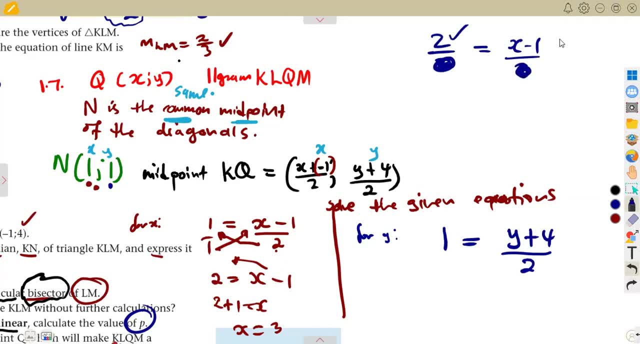 understand that if the denominators are the same also the numerators are are the same so meaning 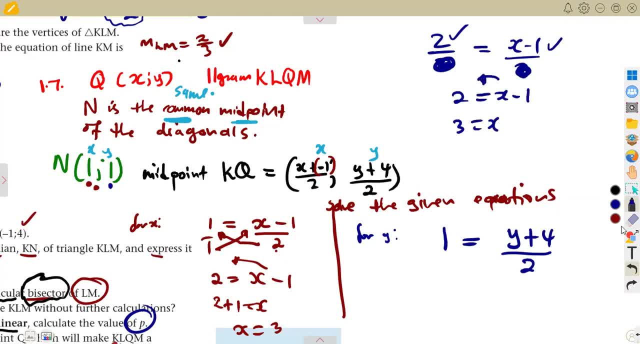 to say i can transpose this and 3 is equal to x just like this part so you could have uh taken it that way or you can just apply 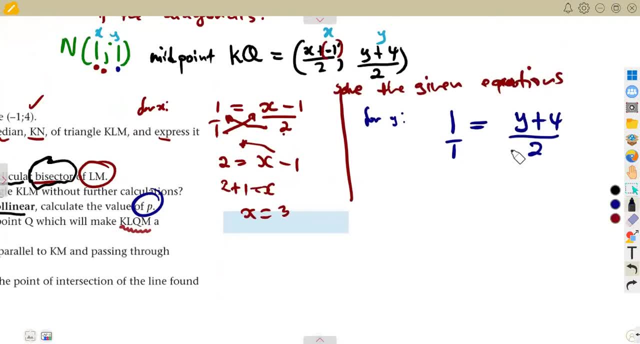 cross multiplication because uh the denominators are the same uh or even if the denominators are the same cross multiplication can be used so 2 times 1 that is 2 is equal to 1 times anything 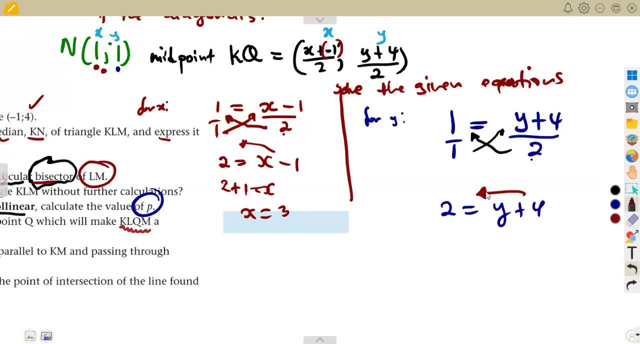 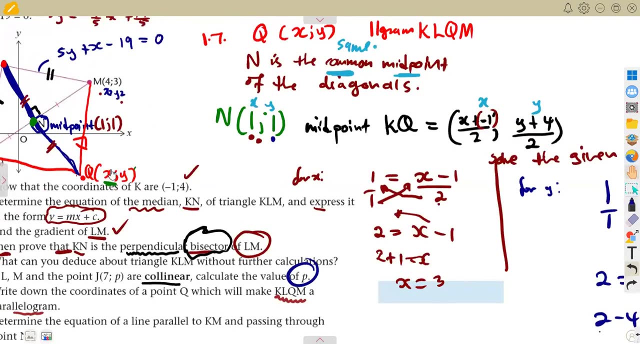 remains as it is so let's transpose the 4 this side it becomes a negative 4 so that's it y is equal to 2 minus 4 which is minus 2 so meaning to say that the point uh q that we do not know 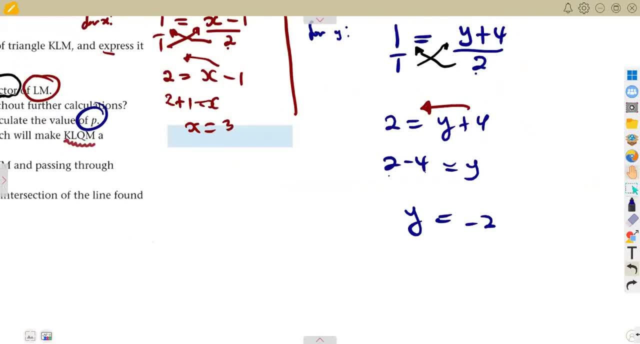 about which is x y is or can be written as x which is 3 and the y value which is minus 2 remember 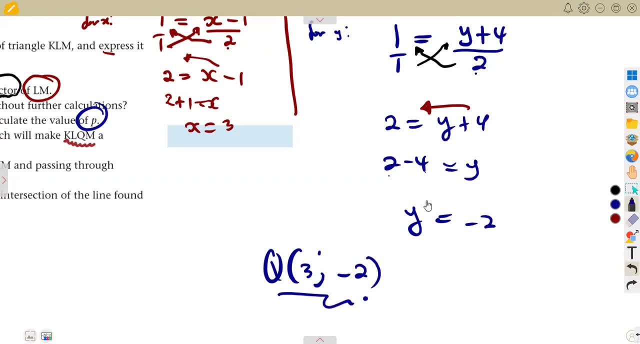 a point always is written in terms of x and y so that is our point q which is 3 minus 2 so this is 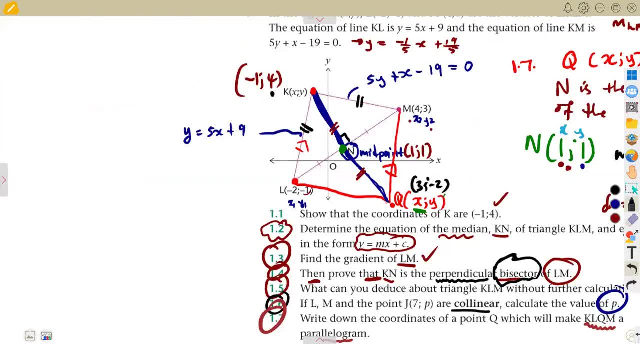 3 uh minus 2 just like that okay so that's how you play around these typical 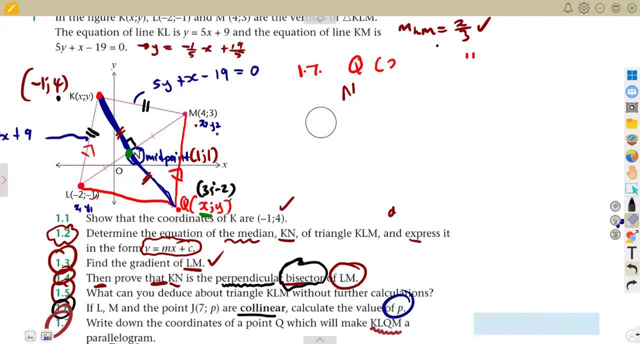 questions yes sometimes you just have a lot to go through uh in your revisions uh to master up 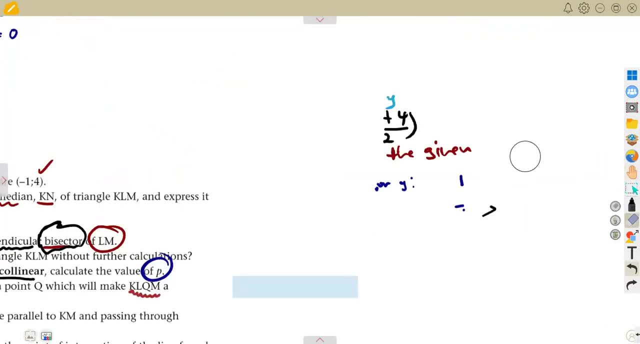 these typical questions uh but as i said maths is not that difficult as long you master up your 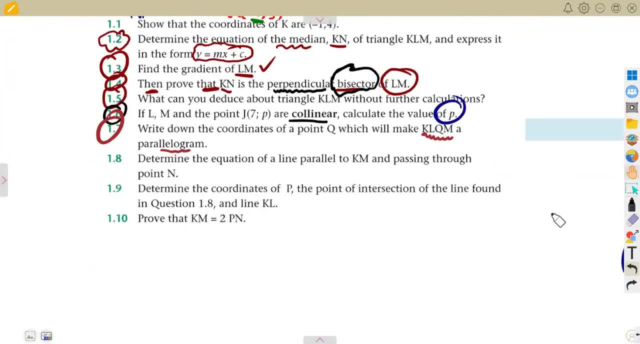 concept then do as many questions as you can you understand this determine the equation on 1.8 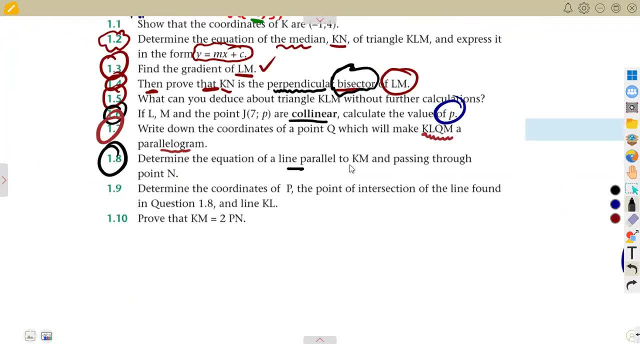 we need to determine the equation of a line parallel to km passing through n 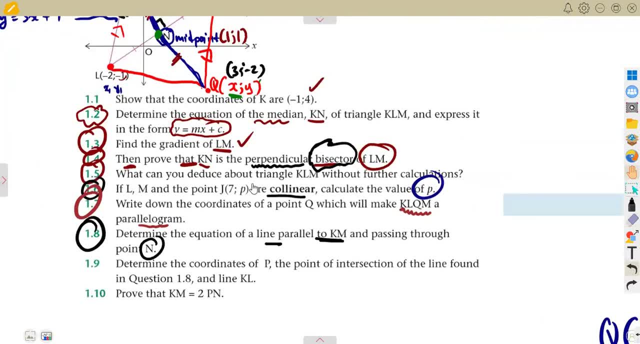 all right it is passing through n parallel to km all right so this is what we need here 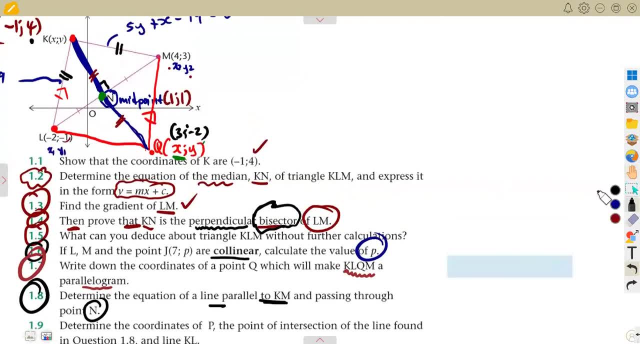 1.8 so if you are to consider this on 1.8 we are given that the line is parallel to kn 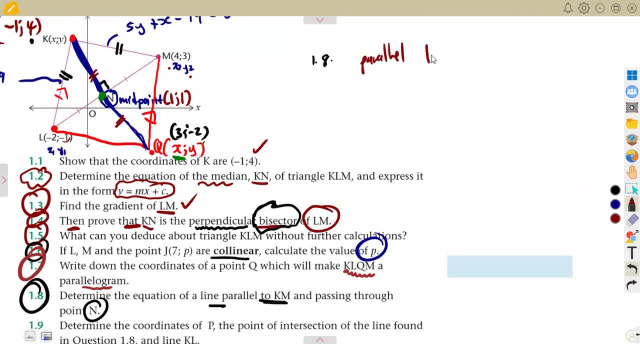 all right parallel to km parallel to km and passes through n we are given where it is going to pass 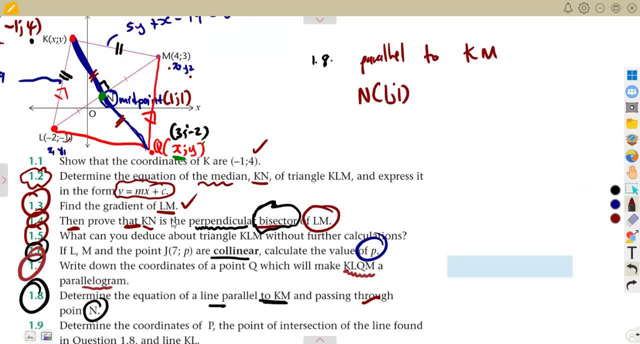 which is n remember n is our midpoint uh that one that we used so what is it that you're going to 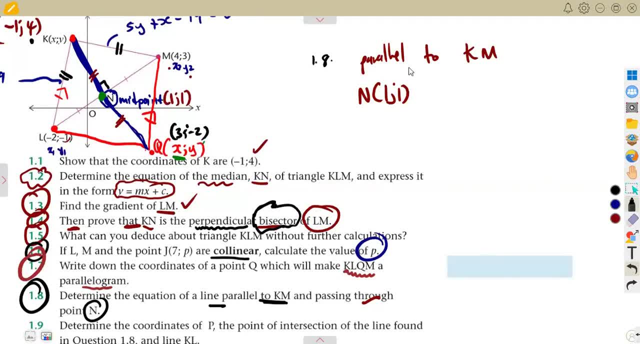 take we need the equation yes but what is that we're going to take from the concept that they 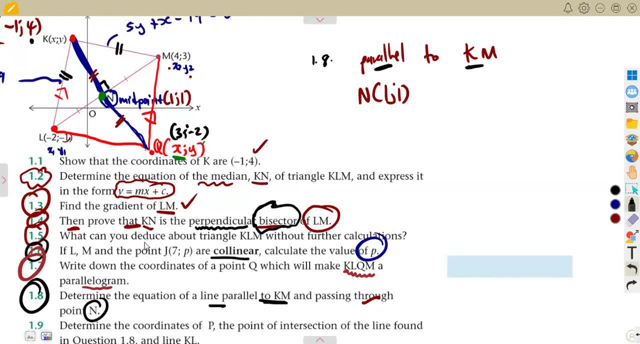 the line is parallel why are why are we given that concept that they are parallel 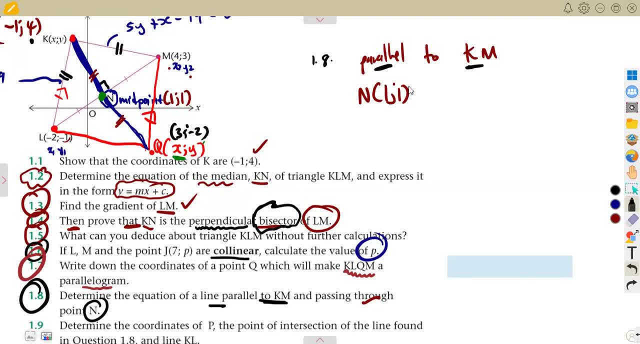 why it is because they know that you are supposed to take the concept that the gradient should be the same the gradient of this line that you want must be equal to the gradient of km 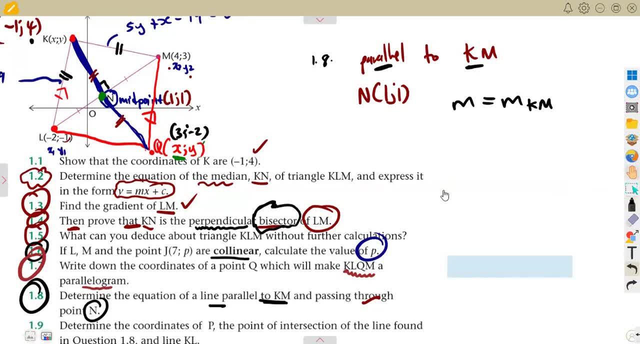 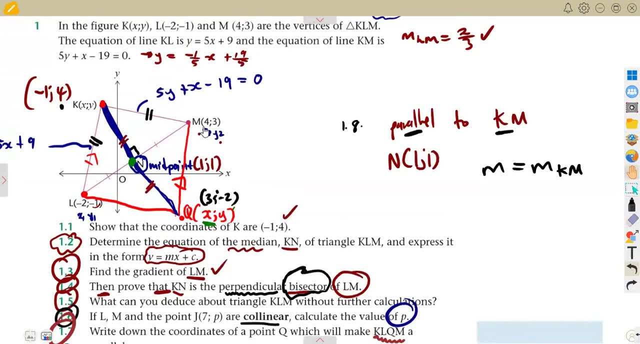 we're having the gradient of km uh that is k to m this one we never calculated its gradient but we can determine the gradient it's either you're going to calculate it or you can take it from the equation of km remember i said the equation of km if you still remember can be written in this format where we made y the subject of the formula so it simply means minus 1 over 5 is our gradient 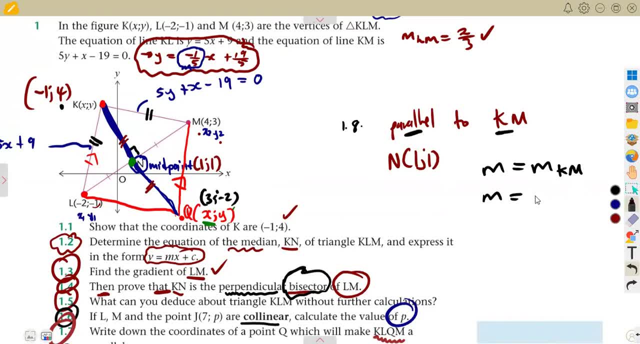 so meaning to say we have the gradient there so you can calculate their points there you can calculate your points i mean from the points if you want uh to verify on that one you can verify from the points which is fine all right 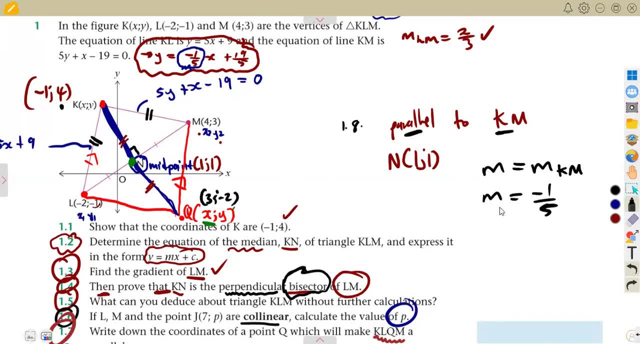 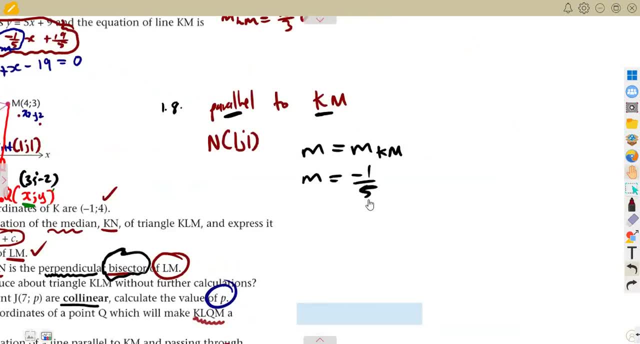 but already this gradient was there from the equation you can tell your gradient is minus 1 over 5 so the gradient is the same so from equation uh concept i don't know which format 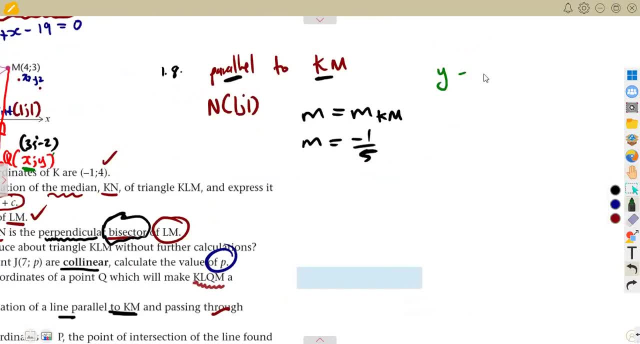 uh but you can determine your equation so i'm going to use y is equal to m x plus c where m is the gradient to be calculated minus 1 over 5 x plus c so to find c which is the y intercept i'm 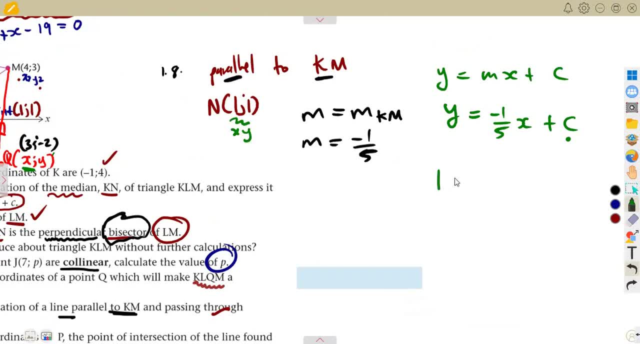 going to set the point that i'm given uh that is x y y is equal to minus 1 over 5 times x which is 1 plus c so that is it uh y is equal to what minus 1 over 5 times 1 that is minus 1 over 5 plus c so let's transpose this is it is going to be a positive 1 plus 1 over 5 that is what you're going to have at the end and that was going to give us 6 over 5 which is equal to c so therefore our equation at the end was going to be equal to uh on this we just have to substitute so this is minus 1 over 5 x plus the c that we calculated which is 6 over 5 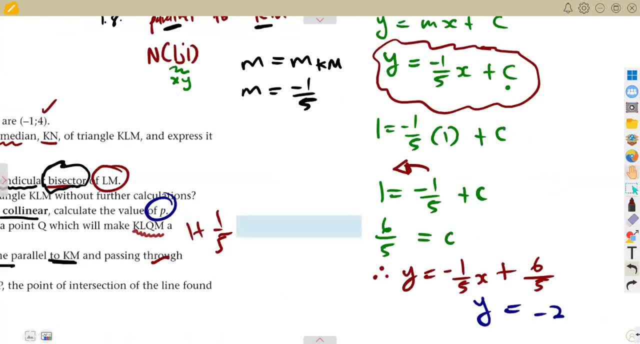 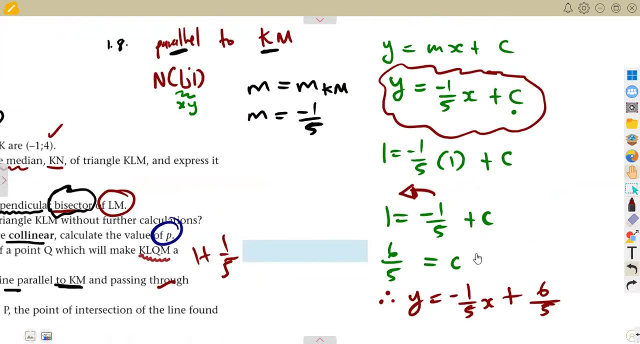 just like that just like that so meaning to say you are ought to be very very careful in your simplification part because any mistake can affect everything as you can see this is from another part anything it can be 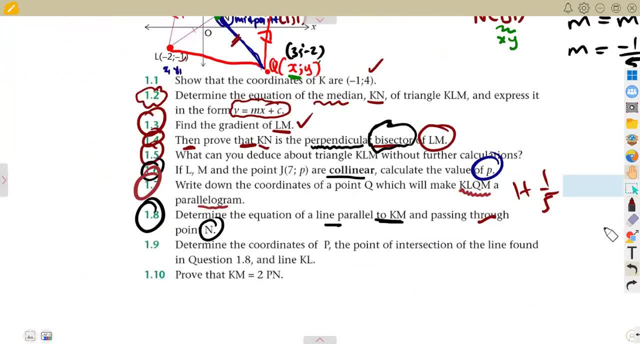 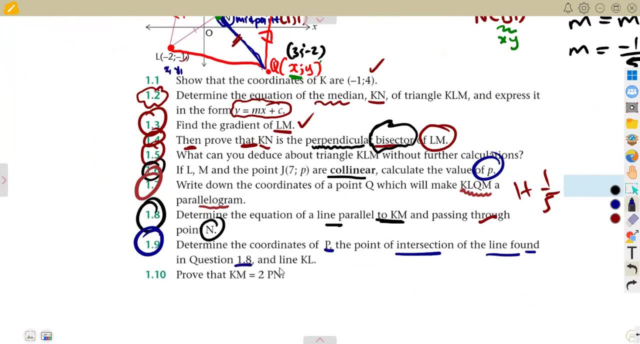 affected so you have to be uh very very careful on how you simplify determine the coordinates of the point of intersection of the line found in ques book 1.8 and the line kel kl the equation of the the point of intersection of the line found in question 1.8 and the line kel kel the equation of the the point of section of the line found in 1.8 1.8 the equation parallel to this all right so that is it there 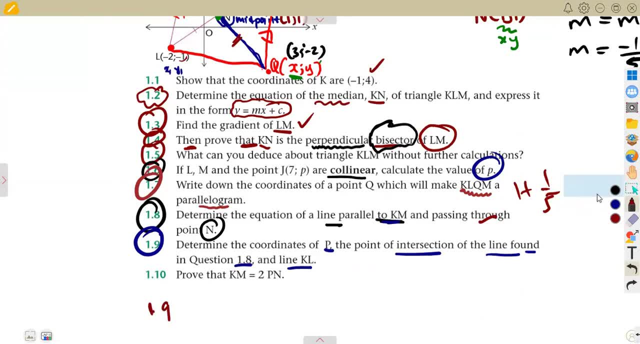 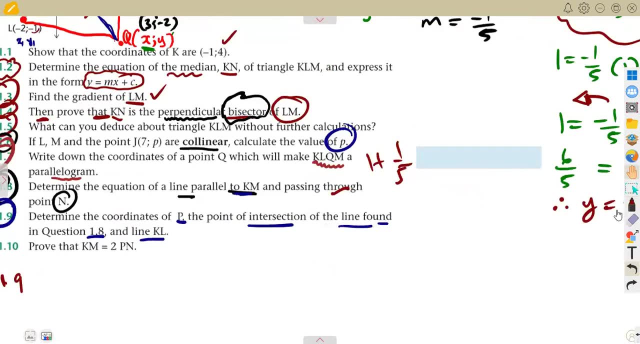 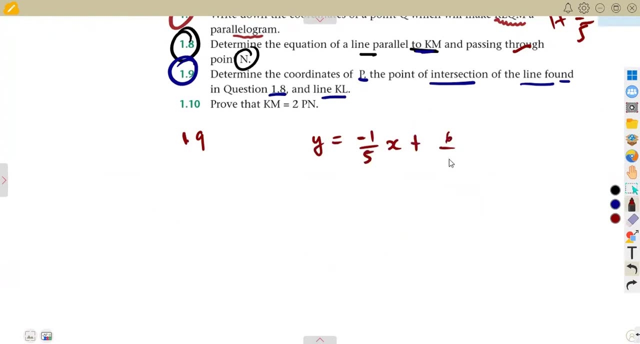 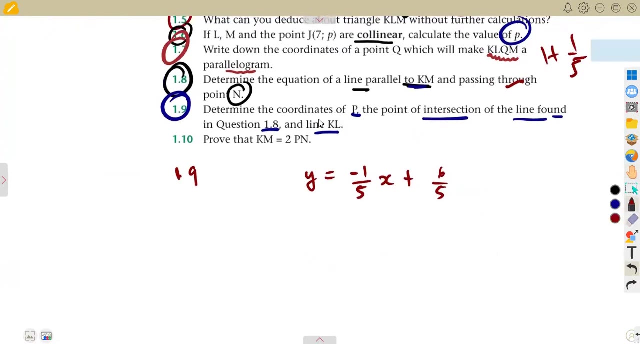 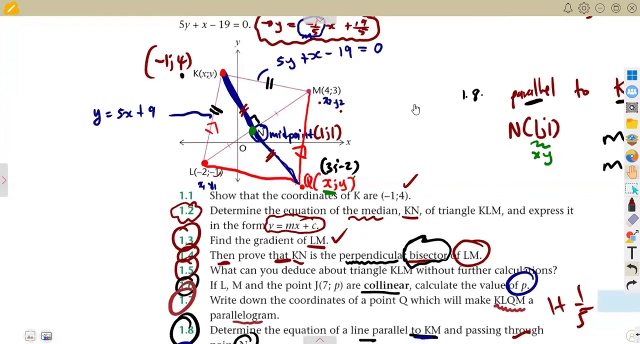 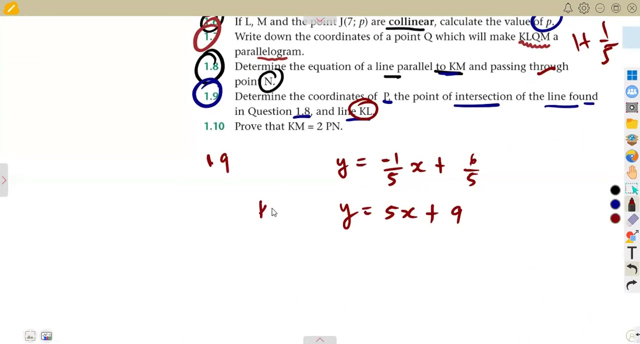 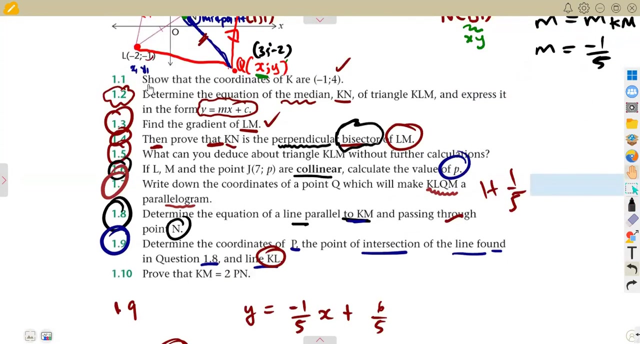 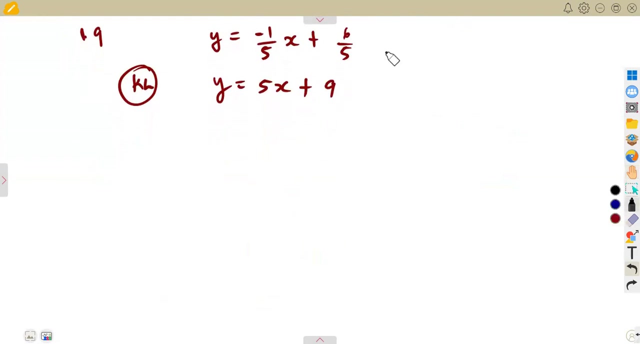 on 1.8 remember we calculated this equation that is the the one that we just calculated right now this is the one y is equal to so i'm just going to rewrite our equation uh y is equal to minus 1 over 5x plus 6 over 5 that was our equation and that line uh so we need the point of intersection of this and the line kl uh kl we have the equation remember for kl this one y is equal to 5x plus 9 so the equation is there y is equal to 5x plus 9 this is the equation of line what uh kl we are already given that equation so i said that whenever you are to calculate the point of intersection just like what happened uh on question 1.1 where we are to show the coordinates of k we calculated that using the point of intersection concept and i said at the point of intersection the two equations are equal so meaning to say at the point of intersection the two functions are equal so we can solve simultaneously the given equations and there we are already given y in terms of x from equation one y in terms of x from equation two so you can simply equate this y and y they're the same if y is equal to this and y they're the same these are the same so you can equate what is 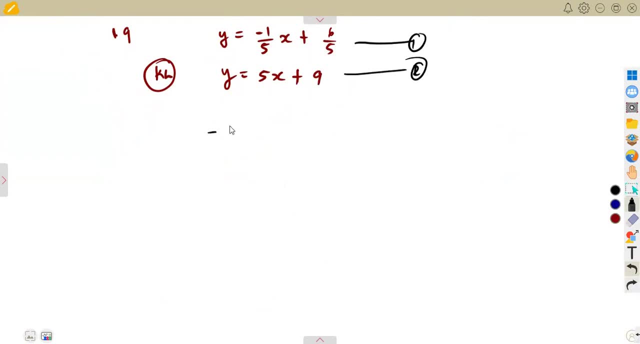 on the right hand side to what is on the right hand side of the other equation so minus 1 over 5x plus 6 over 5 is equal to 5 uh x plus 9 like that so that's you and your equation that's you and your equation so depending with the side that you're going to use let's say i want to maintain the left hand side uh remain with a 6 over 5 transpose the 9 this side is going to be a negative it was a positive so it's going to be a negative so this is equal to on the right hand side i'm already having uh 5x on this right hand side there's already 5x i transpose the minus 1 over 5 to the other side of the equation and i'm going to use this as a of the equation. So it becomes a positive one over five, it was a negative. So on the other side, it will be a positive. So subtracting this, what are we going to have at the end, this will be negative 39 over five, if you simplify properly on your calculator, add five, and one over five, you're going to obtain 26 over five x. So to obtain x, you're simply going to divide by the 26 over five both sides. So you divide by 26 over five both sides, also by 26 over five both sides, that's determining the value of x at the point of intersection. So the x value was going to be minus three over two, if you divide this properly. And since at the point of intersection, the two equations or the two functions are equal at the point of intersection, we can substitute the x 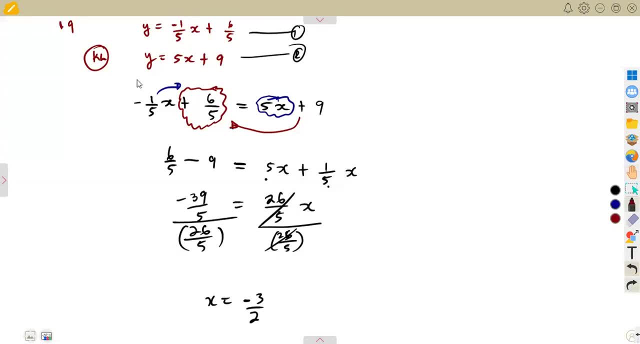 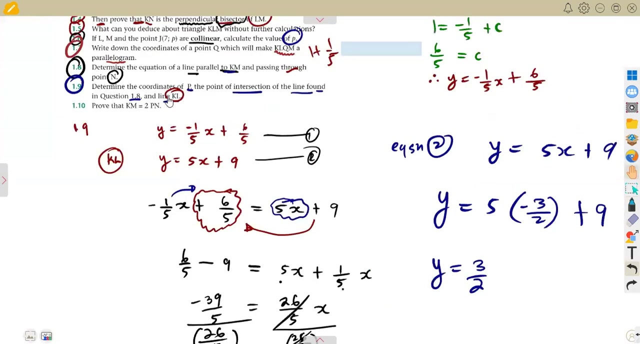 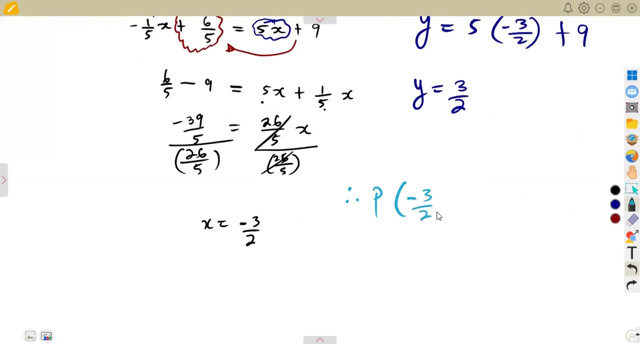 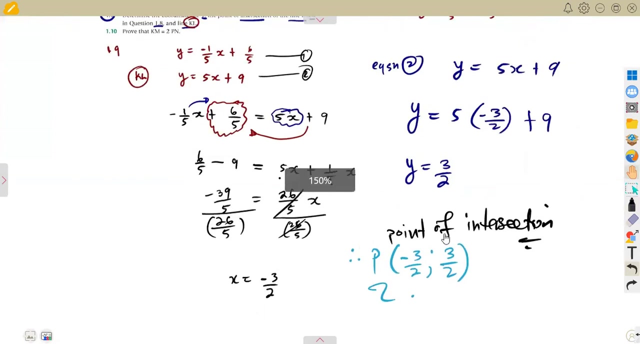 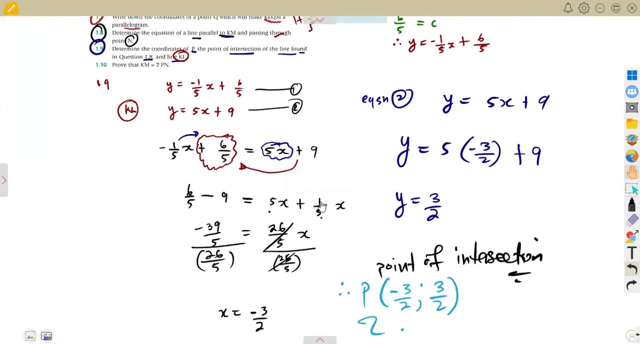 value. That we obtained here in any of the given equation, you're going to substitute in any of the given equation. Alright, so in this case, I'm going to take advantage of equation two, where y is equal to five x plus nine, that's y is equal to five times x, our x value, minus three over two plus nine. Just like that. So meaning to say y is going to be three over two, that's a positive. So therefore, the point of intersection P, remember, P represents the point of intersection, the way that you're given, calculate the coordinates of P, the point of intersection. So P from x, y, x is minus three over two, y, there is three over two. So that's our point of intersection. So that's how you simply work out the point of intersection, you're supposed to be very, very careful in every simplification, solving of equations, as you can see, you're back to those simultaneous equations, you are now working with the simultaneous equations there. 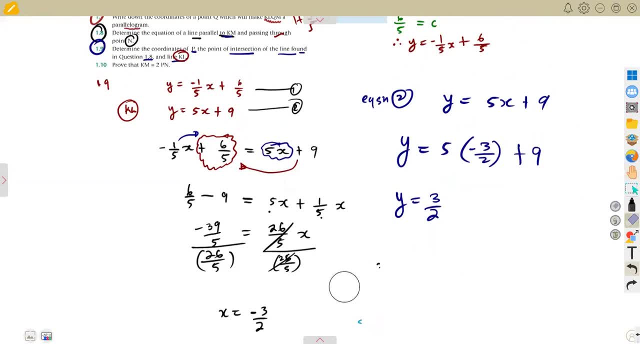 That's it, that's it, you see how they, they play around there. So you just have to be careful. So that's our point P. Remember it, we might need that point. So we have to be very, very careful, we're gonna need that point. If we're going to be very, very careful, we're going to need that point. 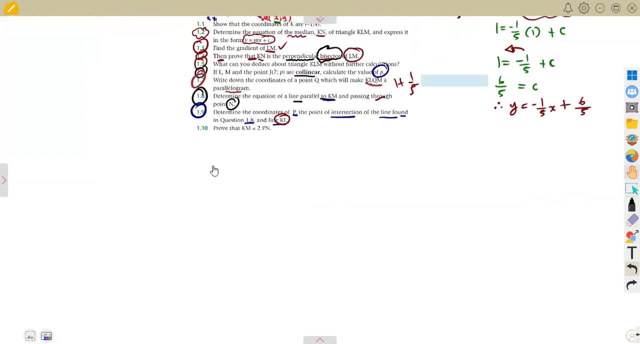 need that point i mean all right then on 1.10 1.10 prove that so there it's a proof a proof you just 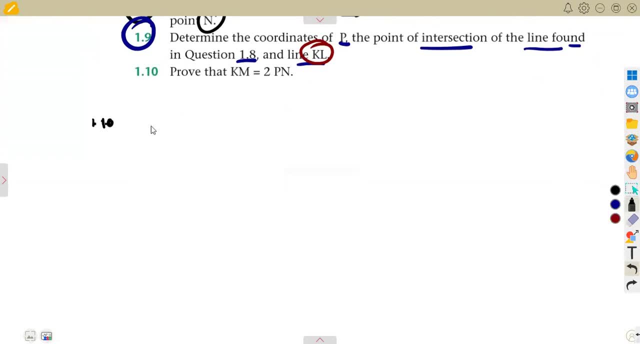 have to calculate when it is like this uh prove that uh km is equal to 2p n this is all about distance this is all about length the length of km the distance from k to m is the same as the 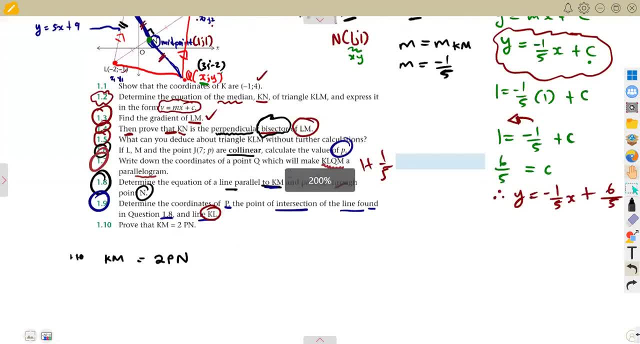 length uh two times length so you just have to calculate because uh that is it guys guys 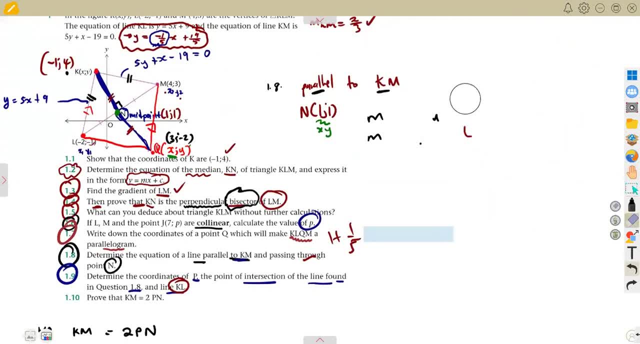 all right no problem so because this video is now too long someone is tired yeah anyways let us see 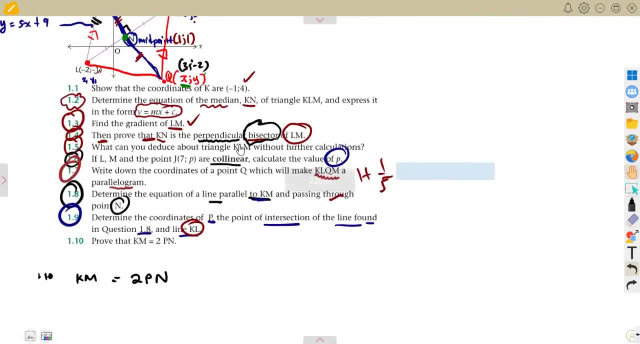 km we have got the point k and m here that is the point k and m so you're going to calculate the 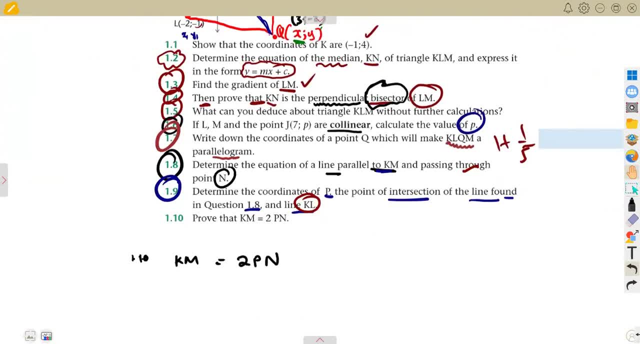 distance of km all right so let me just calculate it to you guys on the diagram 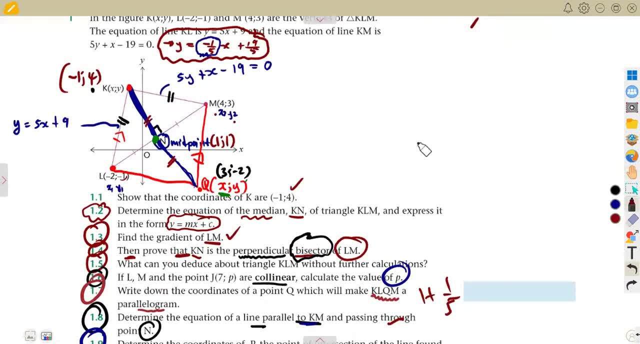 yes somewhere here because so i'm going to answer this question here 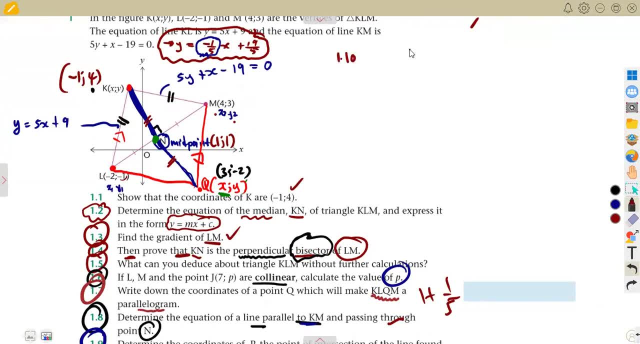 1.10 so remember we want to prove that uh km is equal to 2 times 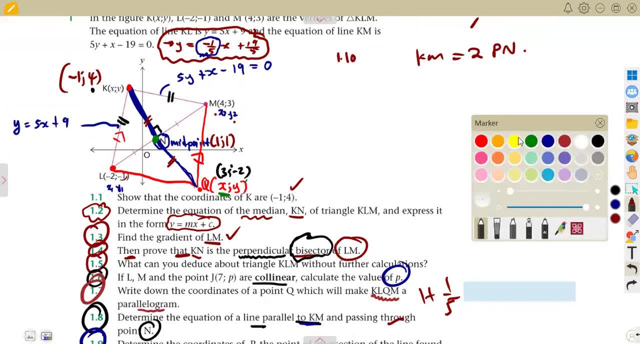 p n so let us just use where we can see uh p uh kn let's start with the length of k and remember 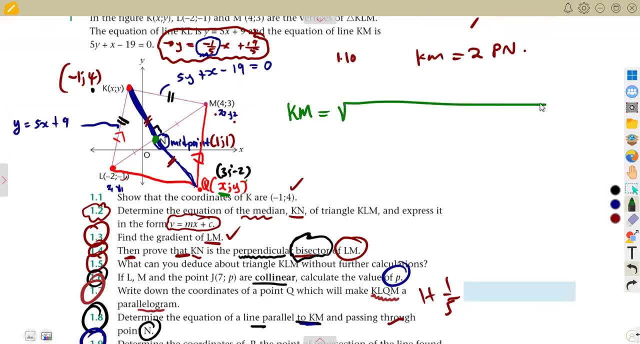 from the distance formula we can calculate this uh x2 minus x1 squared plus y2 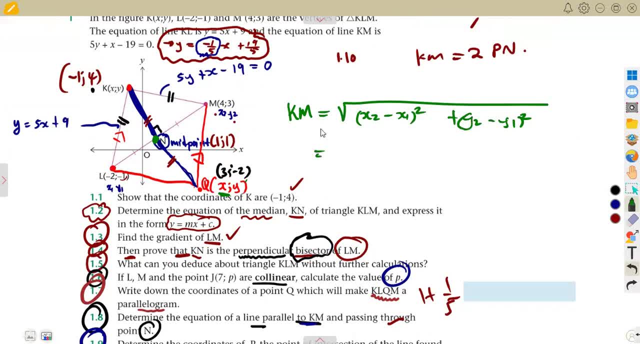 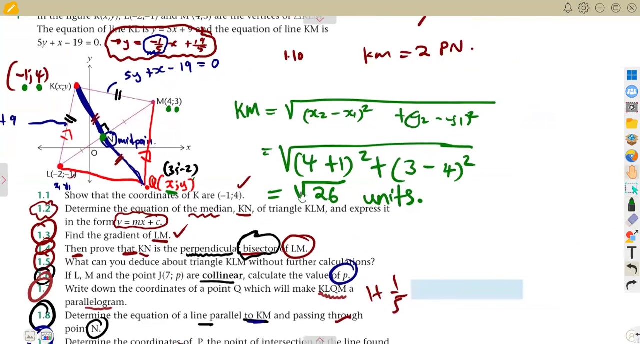 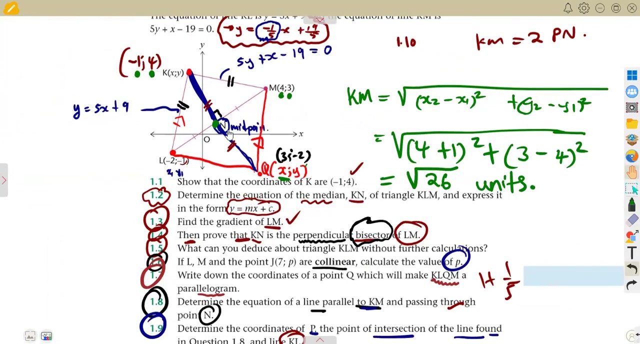 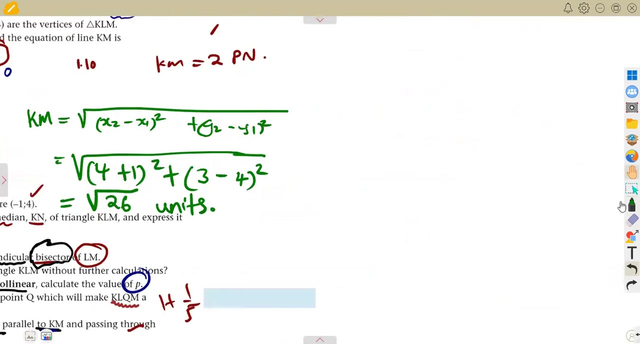 minus y1 squared that is uh depending with the way that you're going to take uh from k and m but what we just need are the x values there so just it's a choice so if you're going to use this as your x2 it's up to you for minus 1 it's up to you the way that you are going to take them uh but that's a 4 minus minus 1 so it's going to be the square root of 4 plus 1 all right 4 for x so it was supposed to be like this 4 minus minus 1 squared so a minus a minus that's a positive so that's 4 plus 1 squared plus y minus y1 so y2 minus y1 that's the y2 value which is at this point m that's 3 minus the y value uh which is a 4 so that's 3 minus 4 squared so that's you and your calculator there just make sure you simplify properly you were you were going to obtain the square root of 26 that is the square root of 26 units then for pn you are going to see that we have got the point n and n here n was the midpoint remember n we calculated that midpoint it was 1 1 i still remember that one so all right also p we calculated p from the previous part that we just calculated now remember our point p was minus 3 2 uh three two that was our midpoint i mean the the point of intersection of those two lines the one 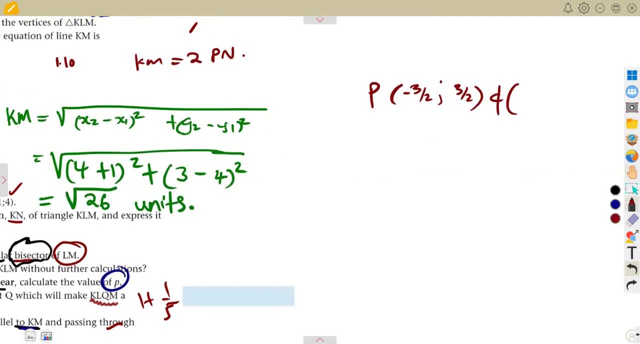 that we solved uh from the previous question and also uh we have got the point any which is the midpoint which is one one remember so we have got two points there so we can calculate the distance 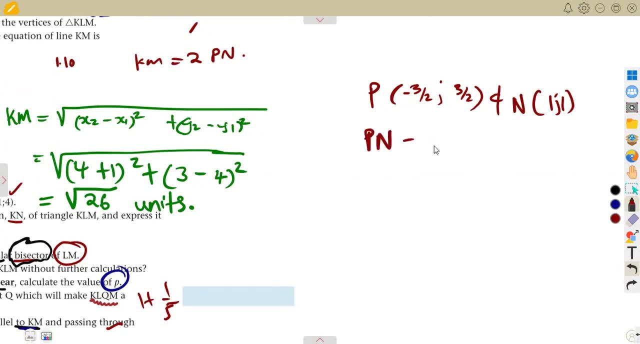 just like this part that we had so p n was gonna be the x value of the second point minus this one so one minus minus that's a plus plus three over two squared plus the y value one minus three over two squared so it's gonna be one minus three over two squared so it's u and the calculator simplify 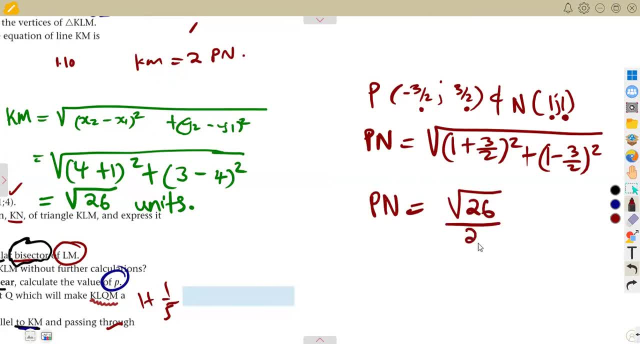 properly it was going to give you the square root of 26 over a 2. so that is the idea there this is square root of 26 over 2. so let's check the relationship this is km which is the square root of 26 and this is p n 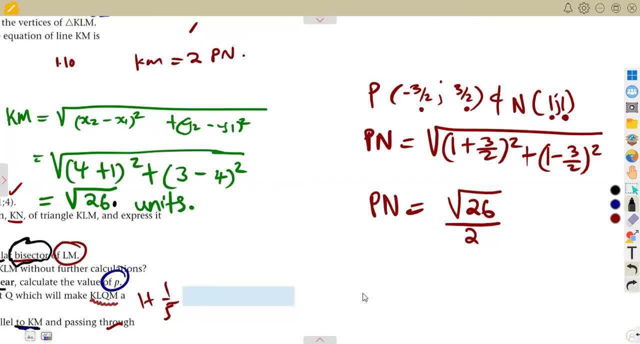 m so if you multiply 2 p m like this 2 times p n that is 2 times p n the square root of 26 over 2 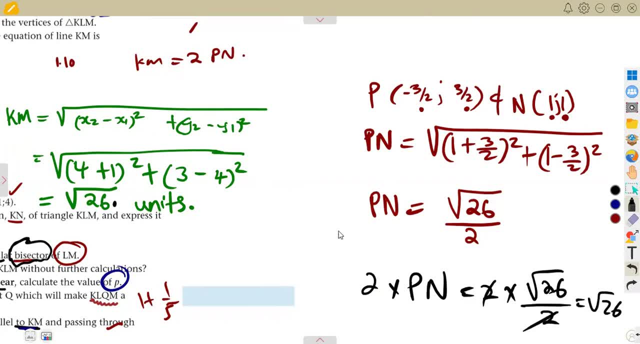 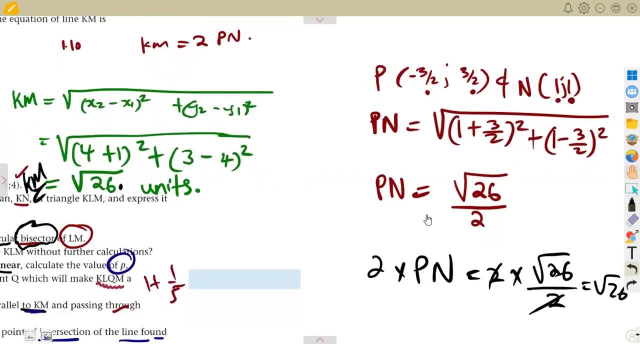 like this this will cancel you get the square root of 26 and the square root of 26 represents what represents km so from this from these values that we can see it simply shows us that truly this km 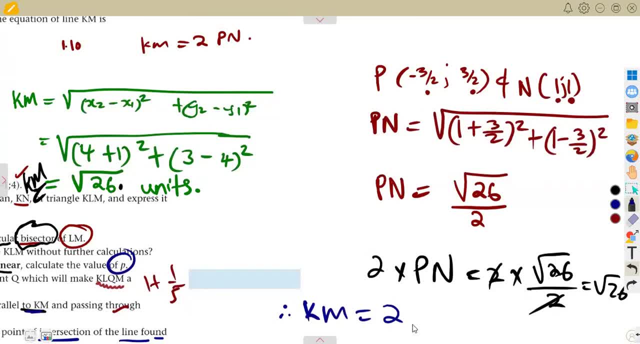 is truly uh two i mean it is two times of what of pn like 2m uh two times pn it gives us km that is the idea there if you can 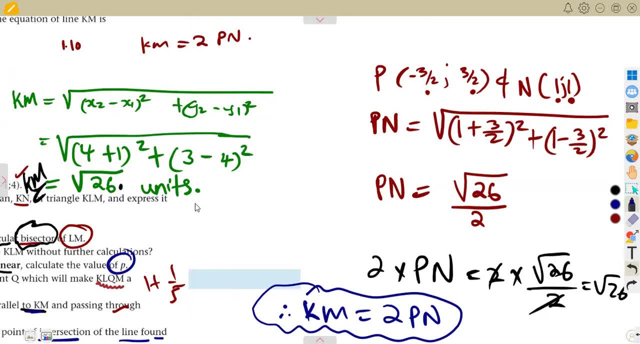 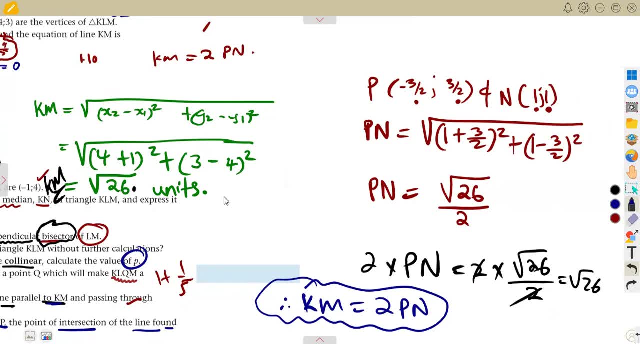 prove from this concept you can see that you substitute this you're gonna get the square root of 26 uh so that is the idea there some of the questions they do not need like uh uh like uh what 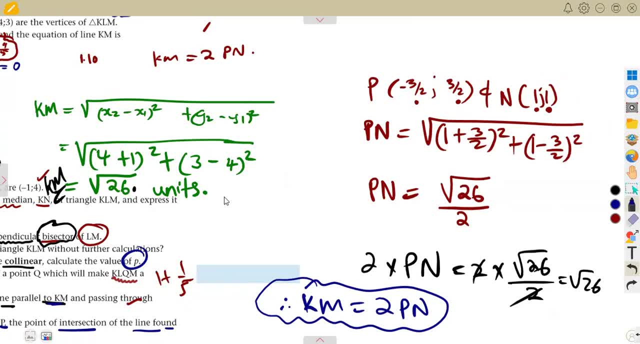 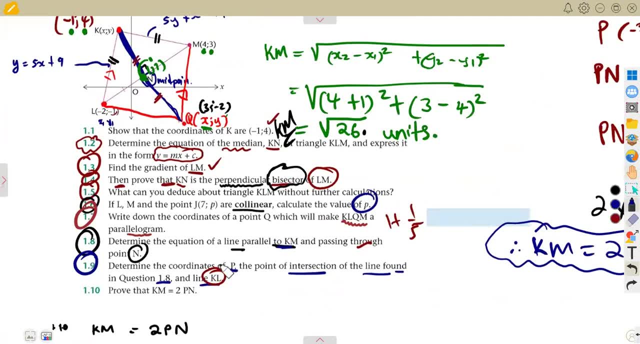 can you say there's no difficult in those questions you just calculate the length as usual you compare those lengths according to the information that you're given maybe it was three times whatever that you'll be given on that 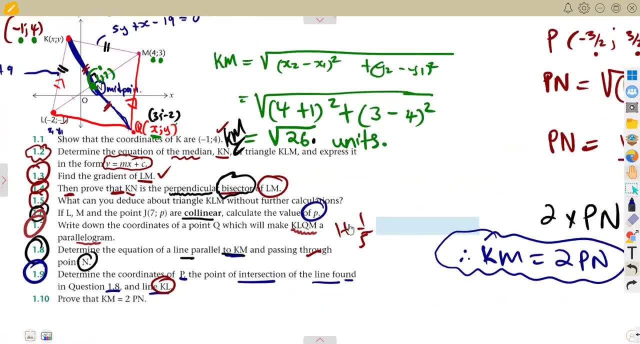 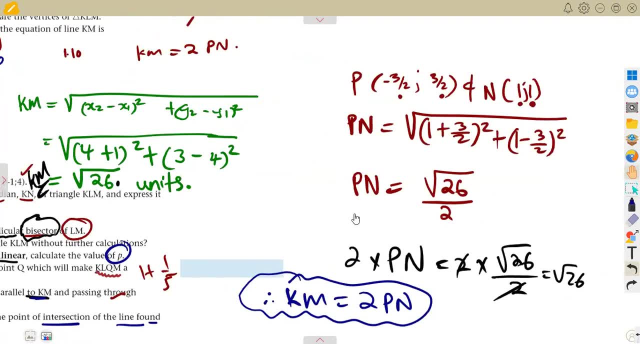 particular question you prove with that condition is it maintaining exactly the condition that you're given if it is maintaining the condition that you're given therefore that's perfect you solve 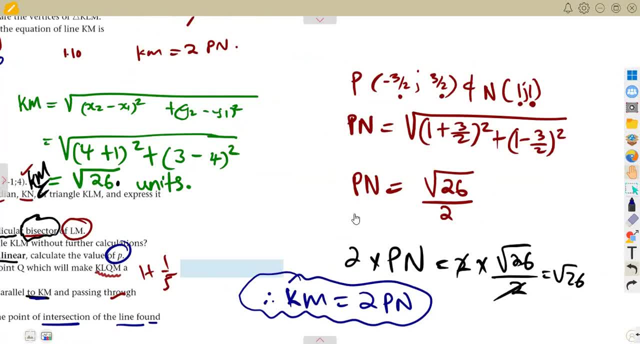 the way that you uh can solve that is to prove a question so more to come from amazon african motives till we meet again